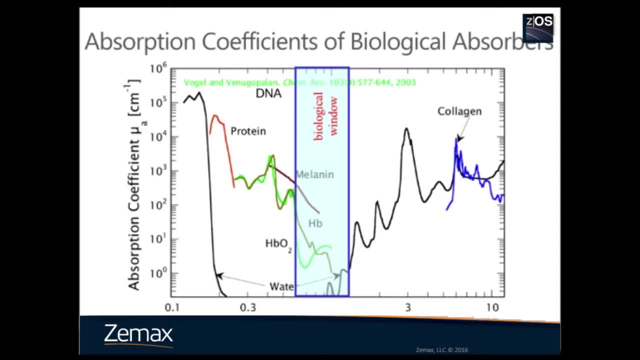 the first few parameters you need to determine when you design an optical system. These figures show the absorption coefficient of different components in a tissue as a function of the wavelength fluctuation. by water in a infrared, by hemoglobin and melanin in a visible, Because of the low 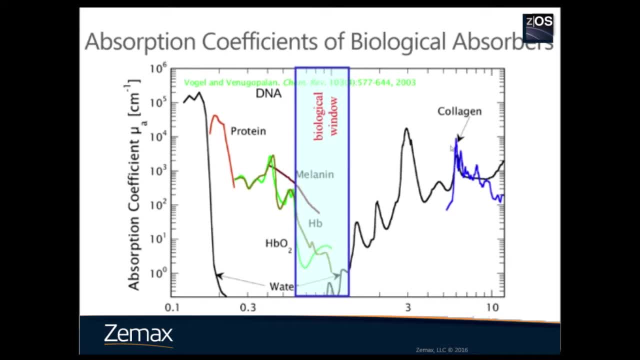 restoration of only one disciple. every life becomes apparent By the way with the civilization of a protein. we preserving these attributes. there is also an identification debility in the label condition freuen angiogen Avec absorption in near-infrared region. This window is often called by biology window. Most of the imaging 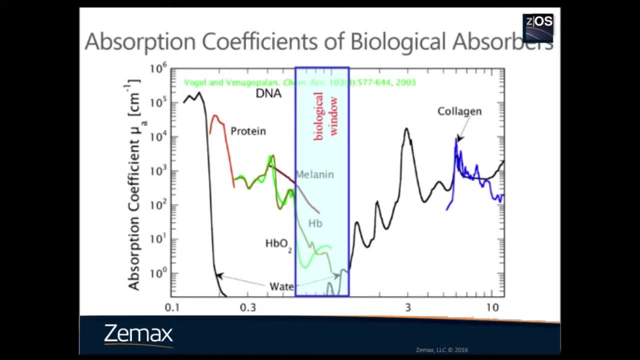 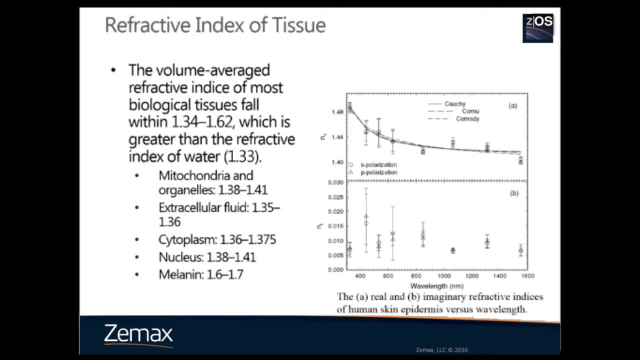 system use a reference in this range visible to near-infrared, for example, 1.5 microns. Tissue is part of the optical system, So we will need to know its reflective index when we design an optic system. Typically we use 1.33, which is similar to the reflective index of. 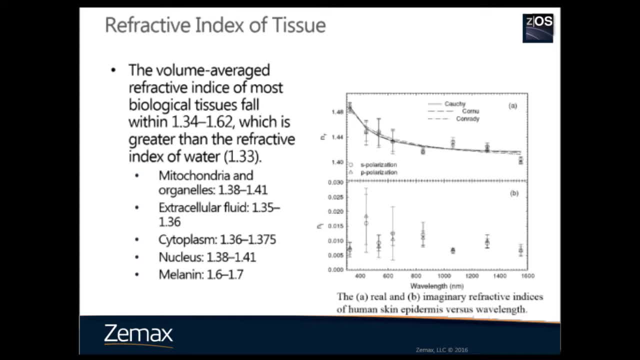 the water as the index of the tissue. However, as you can see from this slide, the reflective index varies a lot from tissue to tissue. For example, Nucleus is about 1.4 and Millennium is about 1.6.. 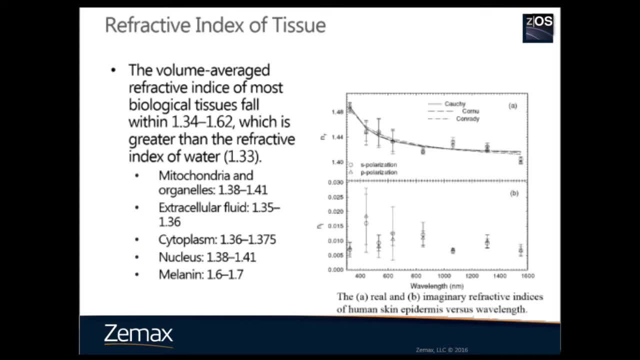 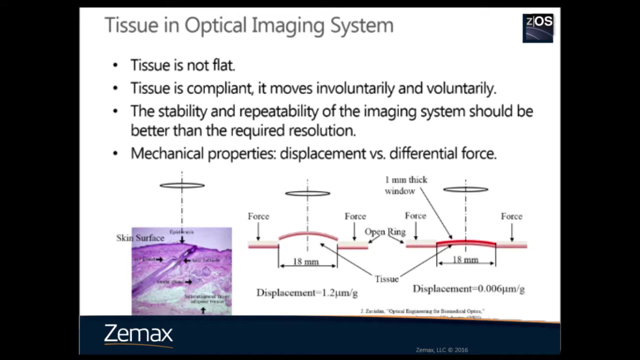 So also I show on this figure that the reflective index is also a function of nerve weightings. So this slide tells us that if you want to design an optical system, you need to know the property of the tissue you want to target. Also, because tissue is in the optical path. 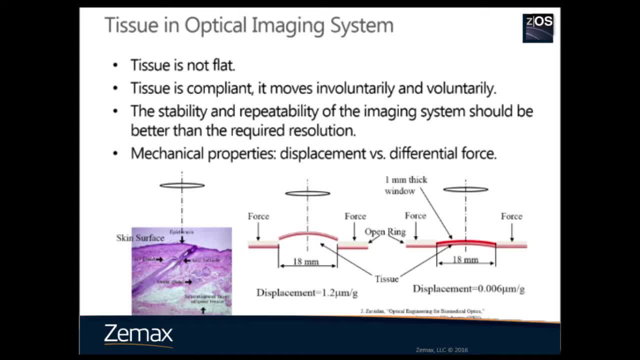 in addition to the reflective index, we need to understand that tissue is not flat. Tissue is a flat object. it is also a non-slip tissue. So tissue is not flat. And tissue is not flat is confined. it moves involuntarily and voluntarily. So if you want to design a 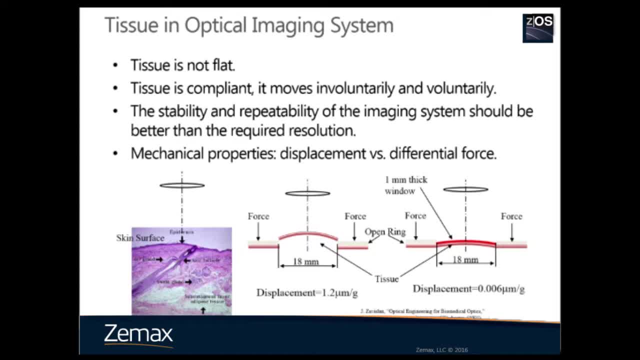 very good system with high resolution. your optic system should be better than the required resolution. Also, if a tube or some part touches the tissue, the tissue will have a displacement. So, as shown in this figure, you can see there is a displacement, Even if you put a window there. if the window is 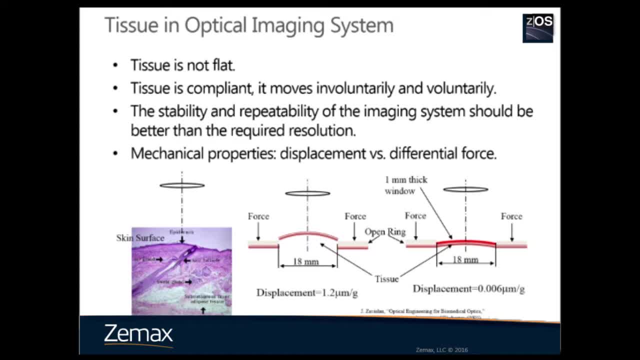 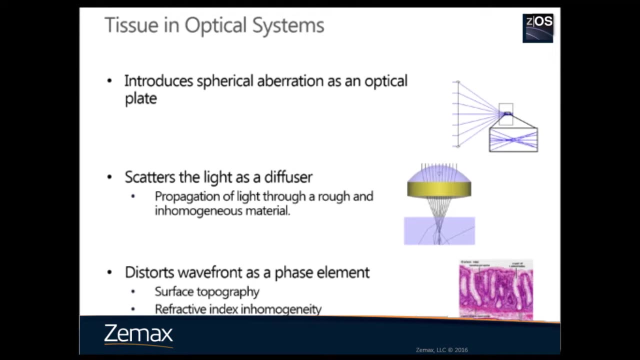 not thick enough, you can still see the slight displacement. So this you will have to consider when designing your optic system. So again, the tissue is part of the optic system, so we need to understand its impact in the system performance, Even if you design a. 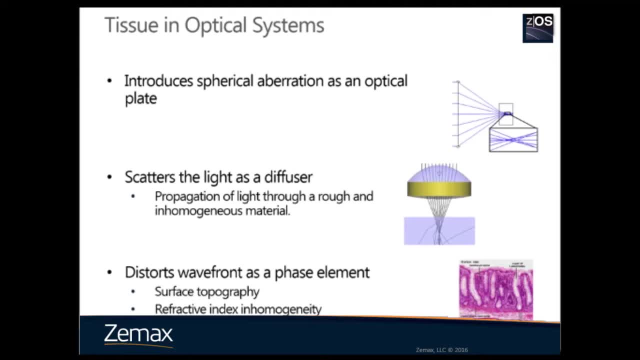 perfect system. when you scan into the tissue, the tissue will introduce the fluid abrasion just like an optic ray. The tissue also scatters the lines, as diffuse as you can see on this figure. So even if you have a great system, 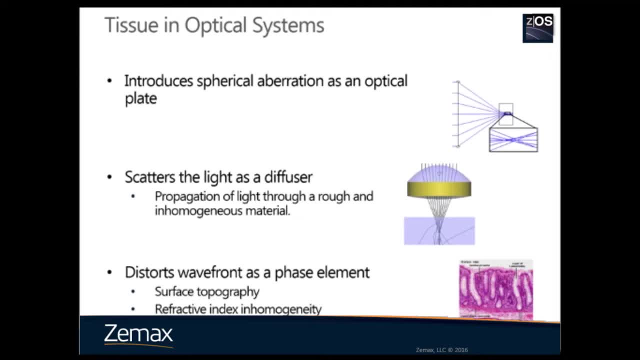 the spot size is much larger due to the scattering Tissue. also, total wavelength is a base element due to the surface topography of the resect index in homogeneity. So that will decrease the system performance. So right now let's discuss the light. 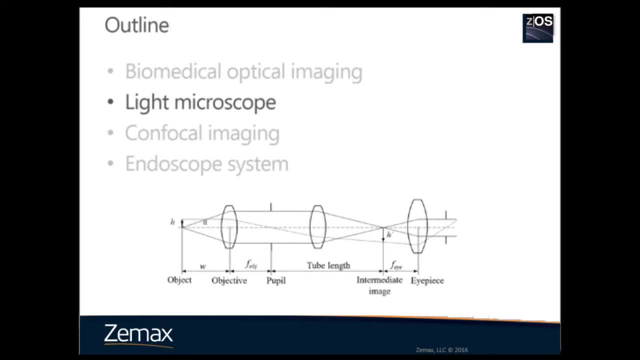 microscopy. I was going to show you some of the ZMesh examples. Microscopy is the most common optic system in biomedical imaging, While microscopy was invented 400 years ago. the principle is the same, The only recent difference between the modern microscope and the traditional microscope 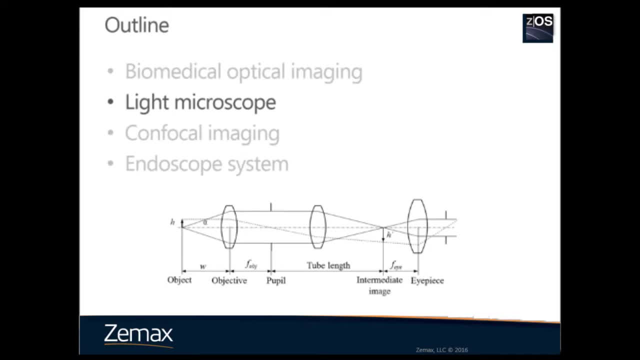 is the objective. Modern objective is infinity conjugate, which means the image is in infinity. So we need to have a to focus the light, focus the image into the intermediate image plane for cameras or IPs And to design an objective. so we need to know the numeric. aperture, fuel rate and temperature, And that's an important feature of this microscope. To design an objective, we need to know the numeric aperture, fuel rate and temperature. So we need to know the numeric aperture, fuel rate and temperature. So we need to know the numeric. 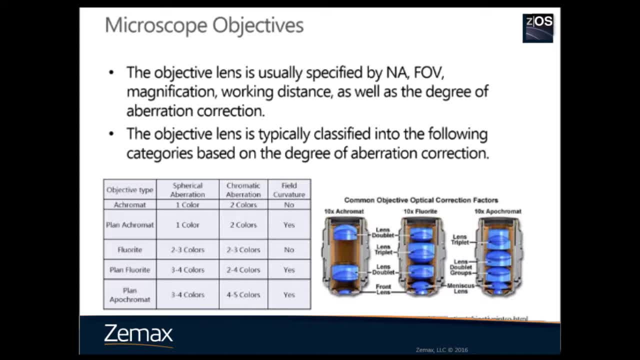 view, walking distance, as well as the degree of the ablation collection. The objectives are grouped into the field categories based on the collection of the ablation: field ablation, chromatic ablation and field curvature. When we need to have a better ablation collection. 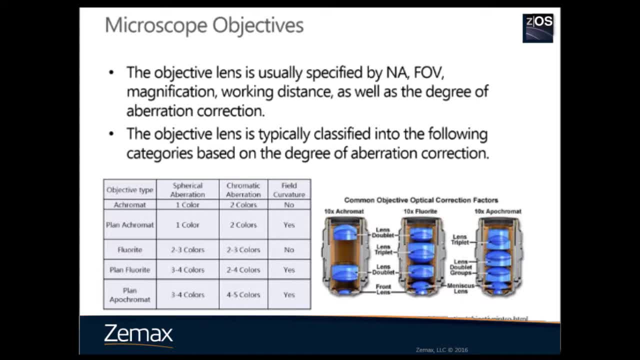 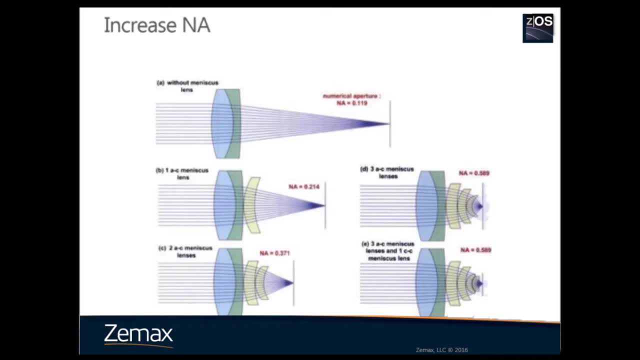 as you can see from these three images, the objectives become more and more complicated. So as a general rule, so if we want to increase the numeric extra, so one way to do it is to add more element in front of the first length. 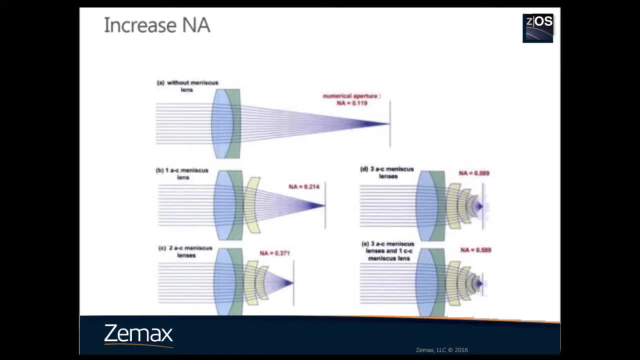 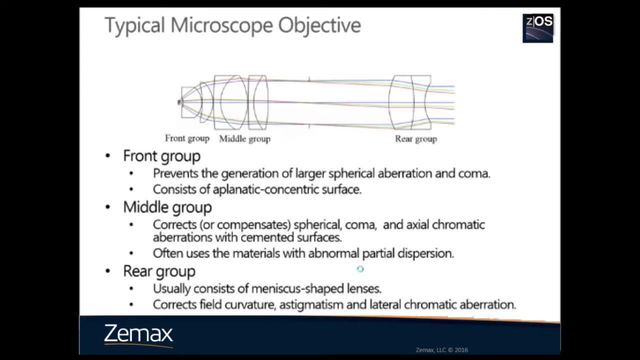 When you add all these elements you need to control the split, ablation and coma. You don't want to have a large split, ablation and coma from this element. So the surface of the element here should meet the condition. So here is a typical macroscope. 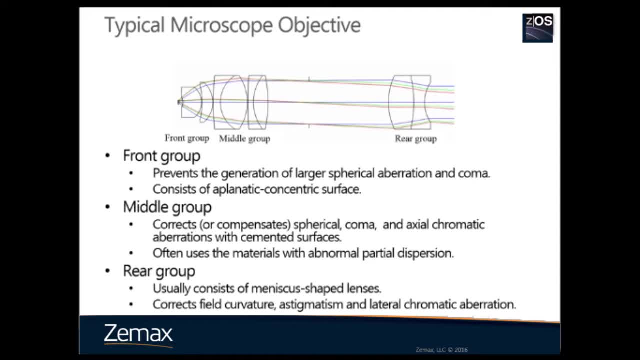 So if we have a single group, each group contributes different to it. So for a real group, so it's most often the use for field curvature correction. So if you don't need to correct the field curvature, you may not need this group. 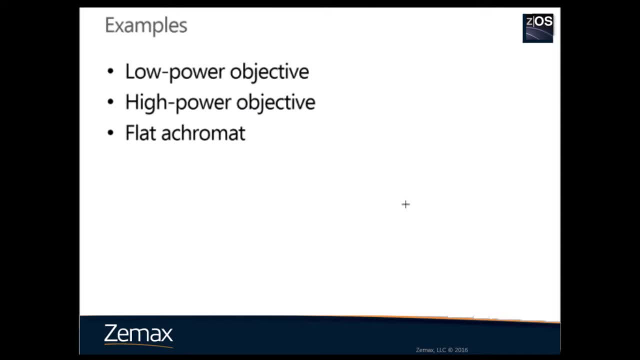 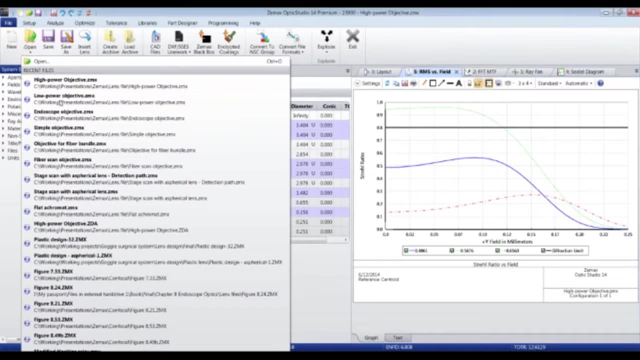 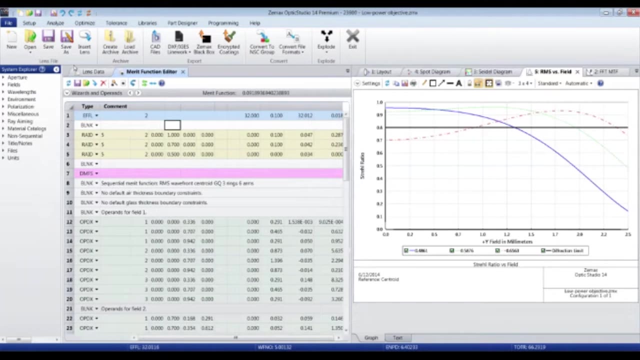 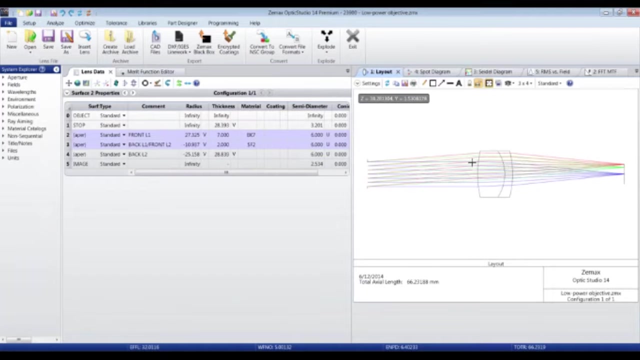 So now let's show some examples. So this is the example of a low-power objective. only a simple doublet is used. So, as you can see, here the aperture is away from the objective and the doublet. The reason is to create a telecentric condition. 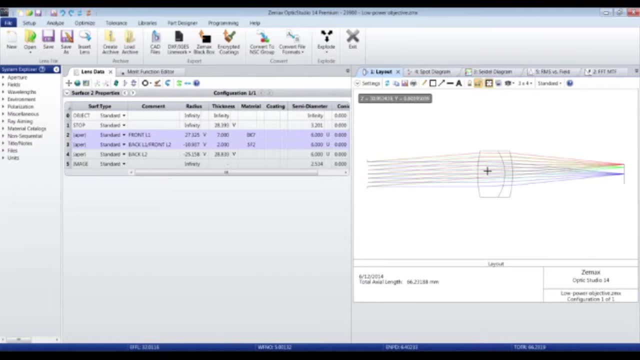 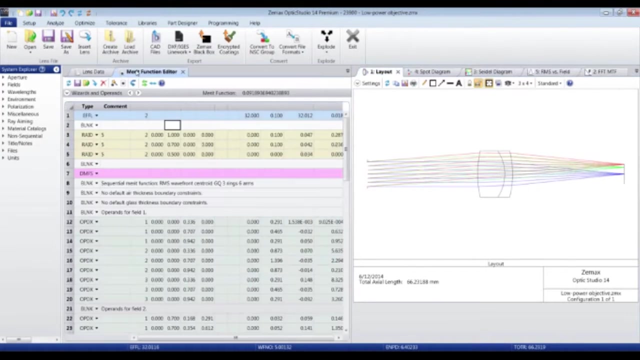 So for all types of microscope objectives, usually a telecentric is not required, But if you want to have a better performance, it's good to have a telecentric in a tissue size In order to control the telecentricity. you can control the chiefly angle. 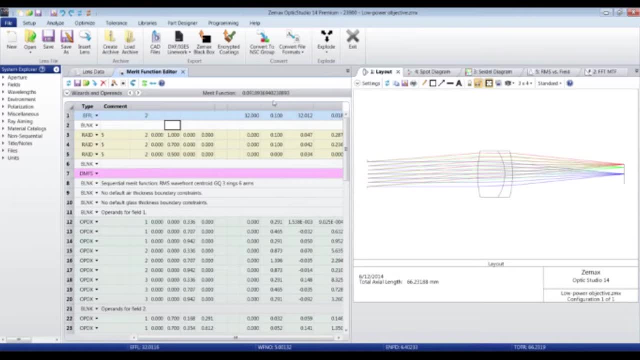 As you can see here, in a many functions you can put a small weight on each angle. You can put a small weight on each opener to control the chiefly angle. As you can see here, for this design the chiefly angle is very small, only less than 0.05 degrees. 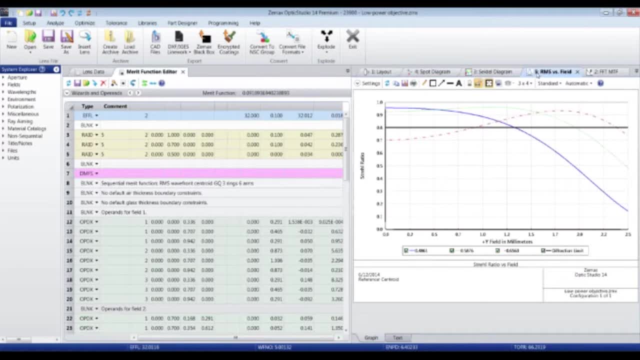 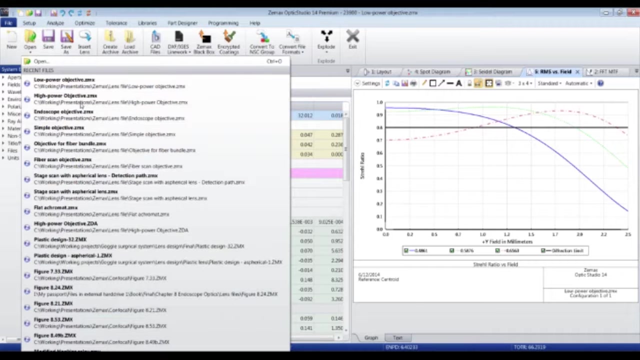 So here is the field curvature, like an RMS ratio. As you can see here it is not a depression limit performance, but you can see for simple objectives that's sufficient. So another example is the high-power objective. So you need to have a high-numeric aperture. 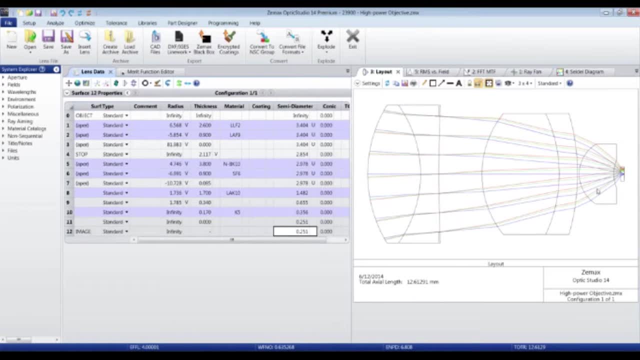 For example, for this example, so you add more elements in front of this doublet, so increase the numeric aperture. So, as I mentioned earlier, so you don't want to, you don't want to, from surface to introduce the large strip, abrasion and coma. 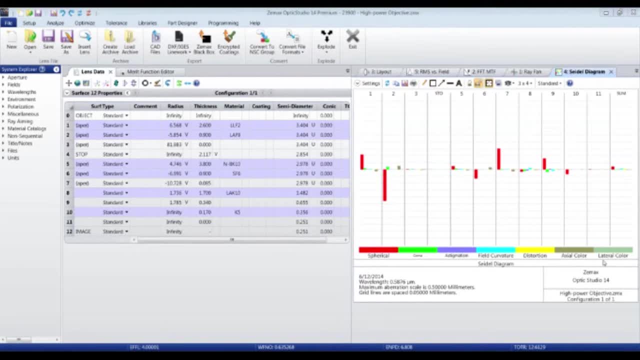 So one way to check the contribution of each surface is from the there diagram. This is a very useful function so you can check the contribution on each surface. So for this example, I also control the chiefly angle. As you can see here it's almost 0.. 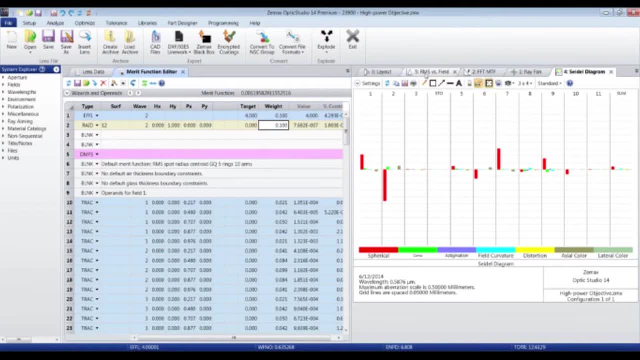 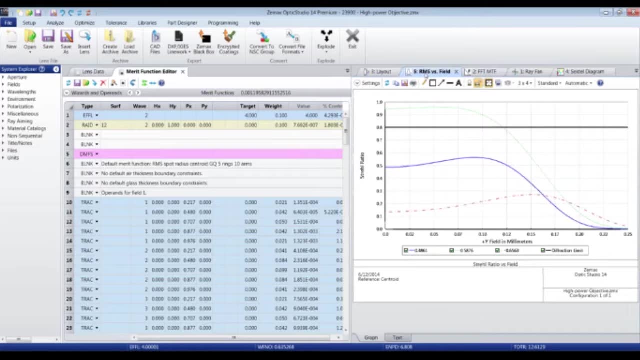 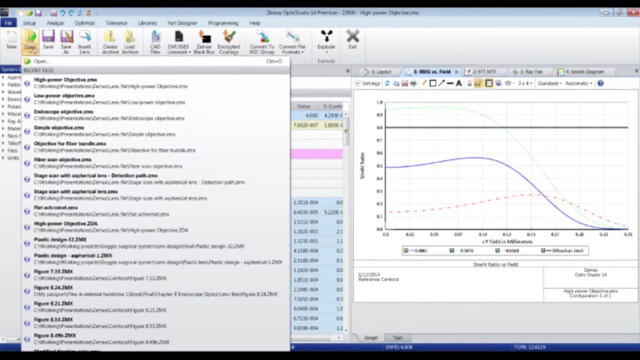 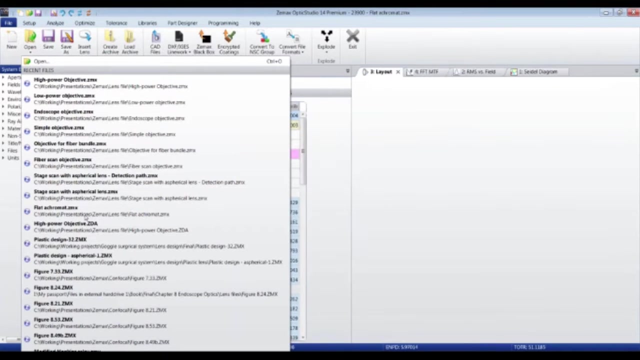 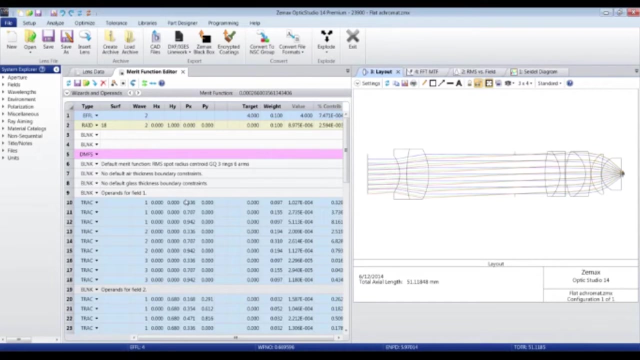 So if you check the RMS ratio, you can see this objective is not where abrasion is not where correct. So you need to further optimize the system. Here is another example. So for previous example, as you can see, so we did not minimize the chromatic abrasion. 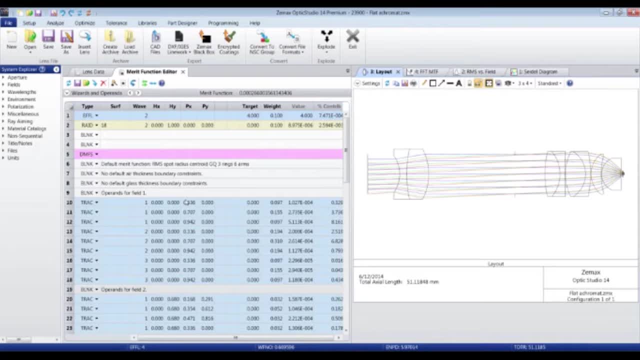 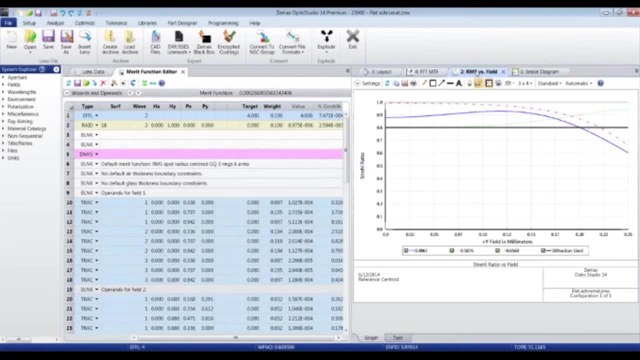 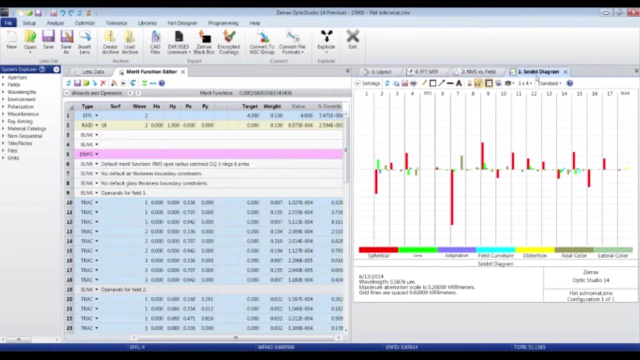 as you can see from the shift of different color. This is another example with the rear group to minimize the field curvature. So you can see clearly from this figure that the performance is very good to have a field curvature very small. Also, you can see that 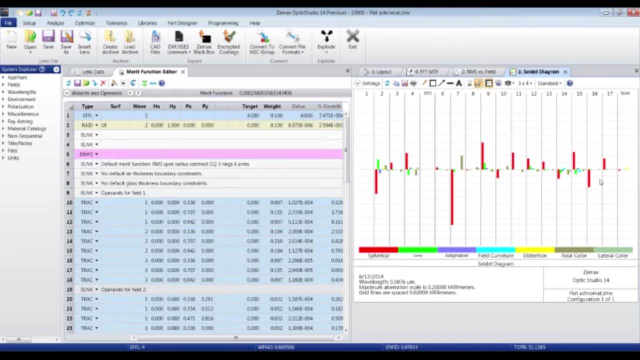 so there the diagram, the contribution of each surface on what application. For example, like split abrasion, you can see that each surface can feel different but they compensate each other, And if you look at MPF, it's pretty good. 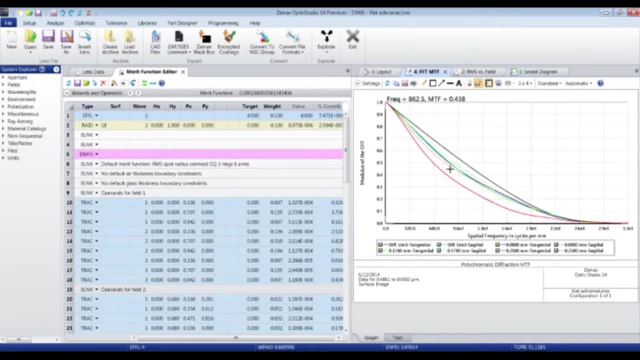 But of course you need to still need to improve it or manufacture. So I also control the shift of the angle for this example. So for the microscope objective, the complexity is determined by your requirement. on the chromatic abrasion control: split abrasion. 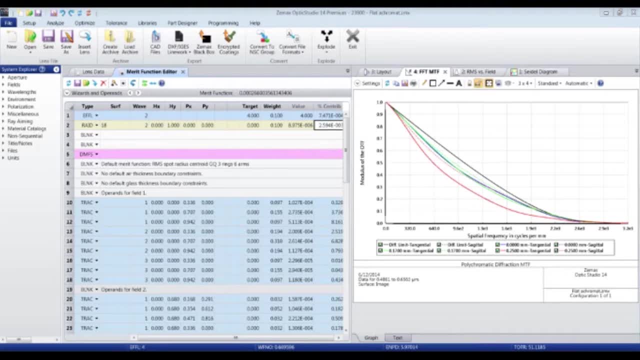 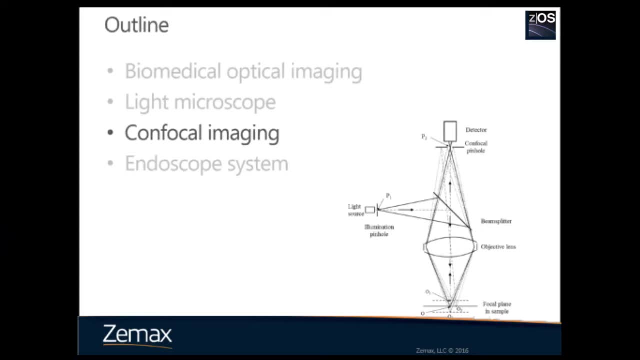 and field curvature. So let's back to the slides. So next topic is the confocal imaging. So, compared to the conventional microscope, the difference is there's a pinhole. There's a pinhole in front of the detector. This pinhole rejects the light. 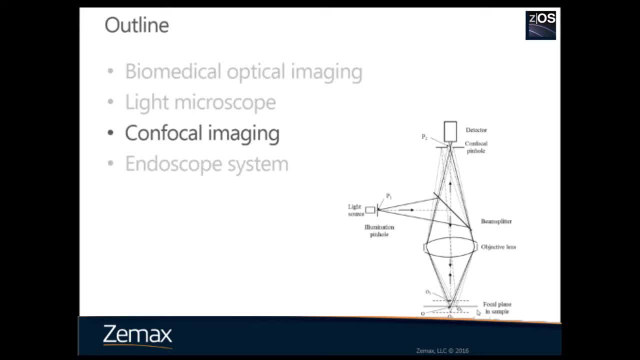 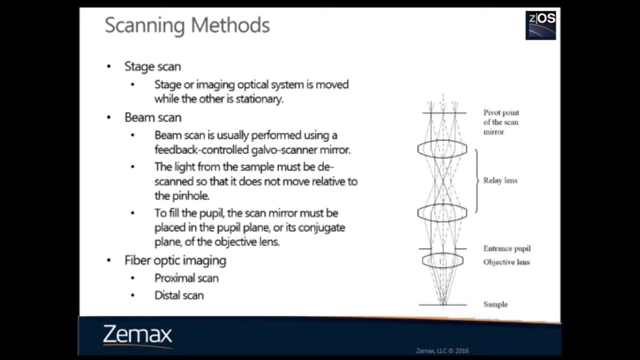 from all our focus objects To achieve a better performance. a pinhole is also needed in the illumination path, But if you use a laser that is not necessary, So because there's a pinhole in front of the detector. so the confocal imaging is a point imaging system. 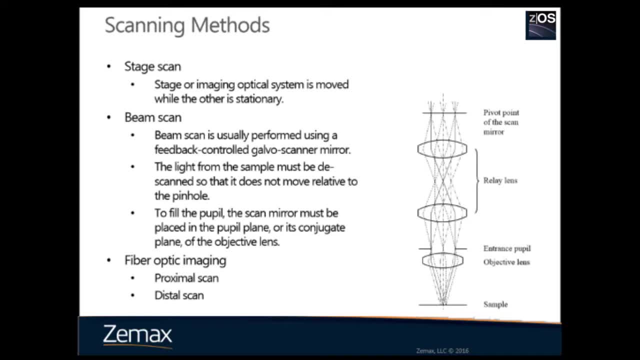 You will need to have a scanning mechanism to create a 2D image or 3D image. So the simplest scanning method is a stage scan. Either a stage or object system is moved. The most commonly used system is a beam scan system. 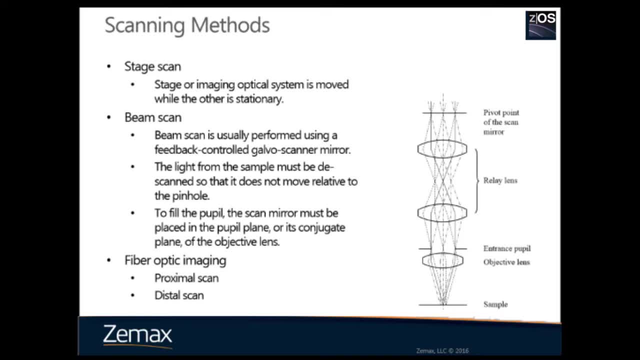 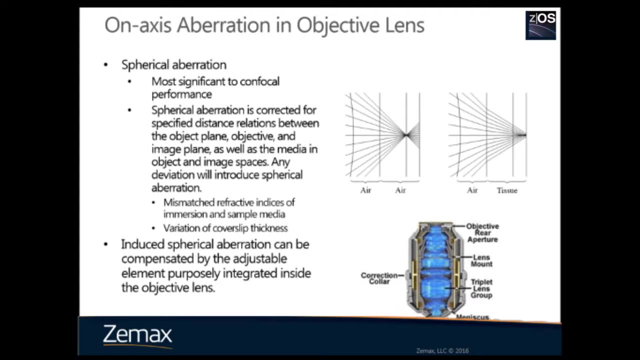 So use a scanner to scan the focus across the sample. Fibro-optic scan is also an option, especially in endoscopes. So what is the requirement on an imaging system? Phylic ablation is always the first ablation you need to consider. 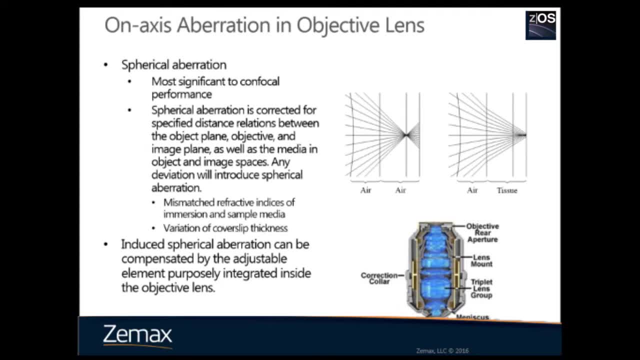 It is an on-axis ablation. You have to minimize for all scanning mechanisms, So also phylic ablation. you have to be very careful, because even you have a perfect design but if you don't consider the tissue thickness and the refractive index, 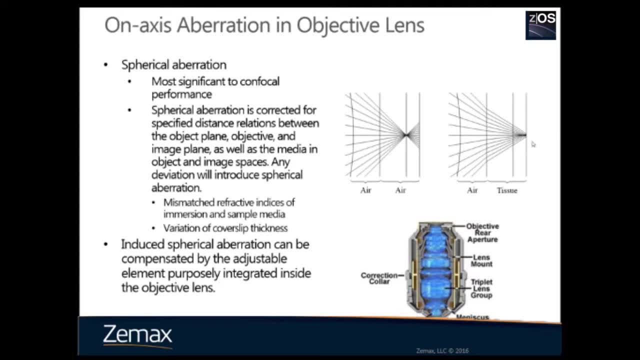 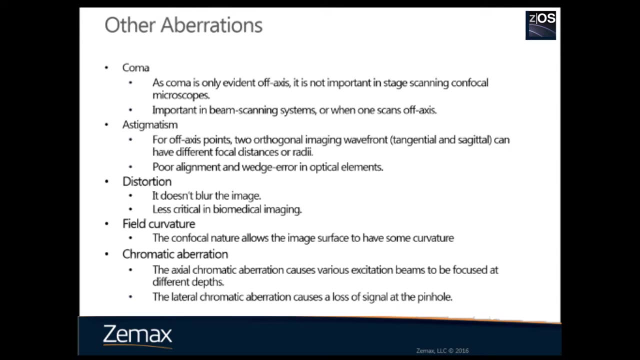 when you scan into the tissue and this tissue will introduce the phylic ablation, as you can see here. This is, for example, your object design as a perfect system in the air, But when you scan inside the tissue, you can see the phylic ablation. 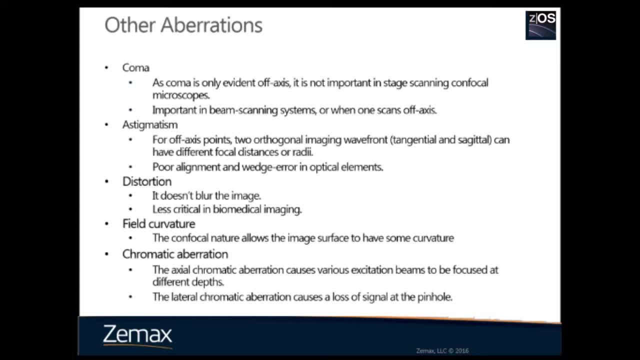 Sarcoma, ischemic sin distortion and field curvature are off-axis ablation, So the correction highly depends on your application. If your system is a stage scan, so you don't need to consider these four types of ablation, But if it is off-axis scan, 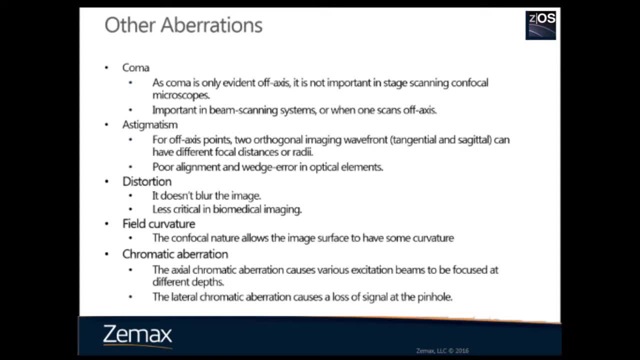 with some bin scan or bubble scan. you need to minimize each of them. The distortion is very different, So it doesn't allow the imaging. So it is less critical in tissue imaging because tissue, as we discussed it, is compliant, so it moves. 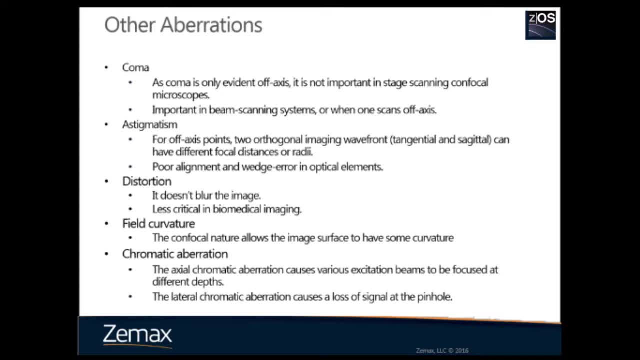 But if tissue is fixed on a slide, then you need to minimize your distortion. Similarly, the field curvature If you have tissue imaging during a surgery or small animal imaging, so field curvature is not necessary to reduce to a very small level As long as the curvature is set. 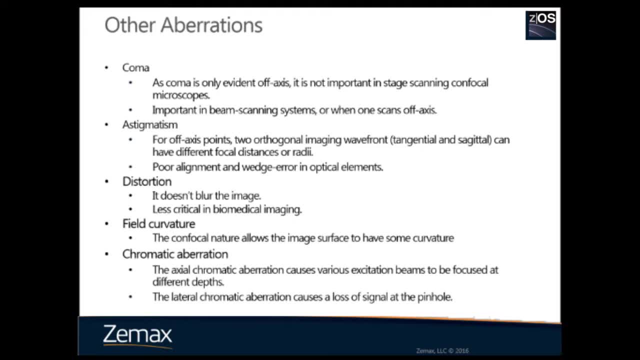 it's smaller than your depth of field. But if the tissue is fixed on a slide and your application is for this, then you have to minimize your field curvature because at that time the tissue doesn't move: Chromatic ablation. so for a stage scan. 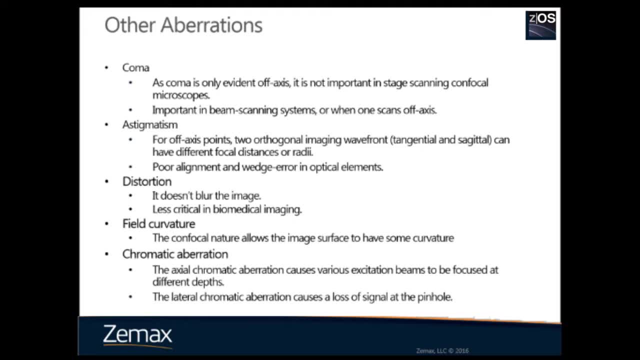 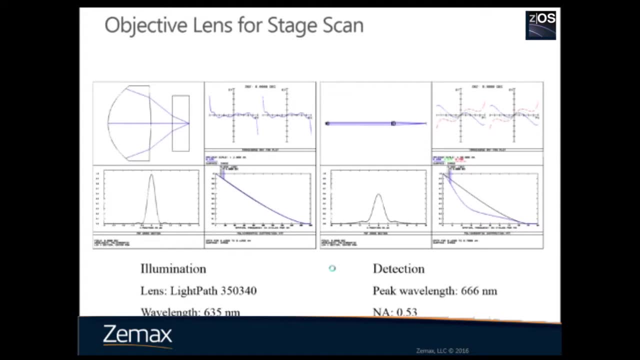 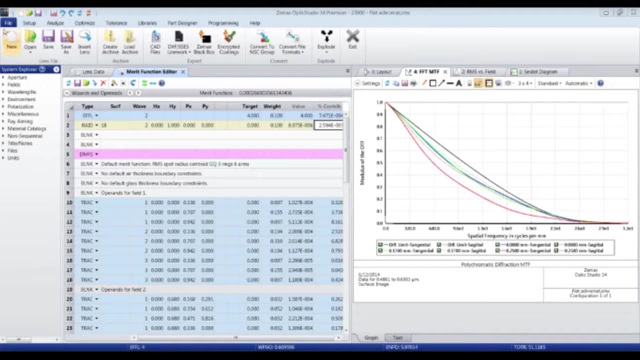 you only need to minimize the actual chromatic ablation. But for bin scan or bubble scan, you need to minimize the lateral chromatic ablation. So here is one of the examples. So let's go to the light source, Let's go to the rematch. 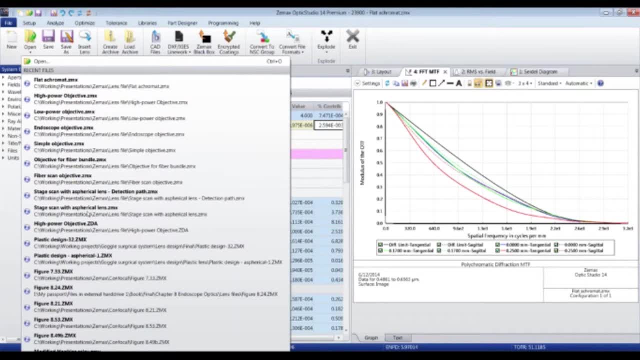 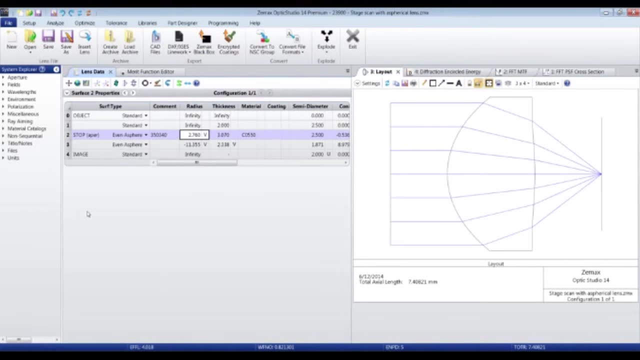 Here is the stage scan for the object for stage scan. So it is a 3D objective. So I'm just going to use that for a comfortable imaging application. So, as you can see here, this is on a 286 surface. It's very simple. 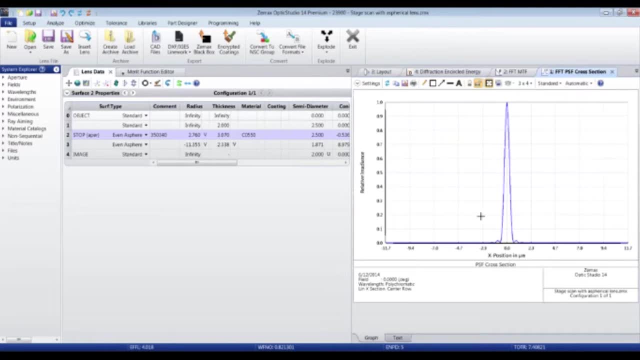 So if you look at the function you can see it has a very good performance. So one unit of visual you can use in here is the in-cycle image, So you know how much light is with how much energy within certain size, especially in the detection path. 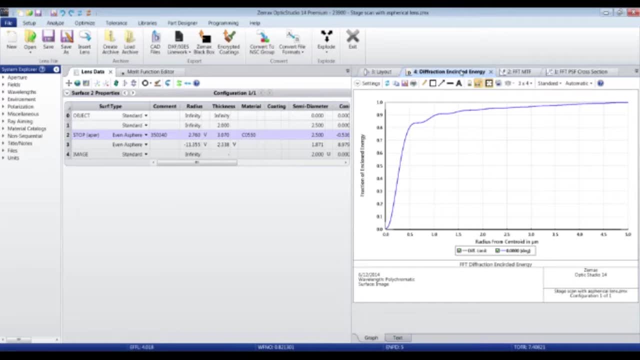 So I will discuss in next example. So for this one only works for, for example, for focal correlation imaging. So excitation at 635, you can have a very good, you know, focal point, a very small focal point. 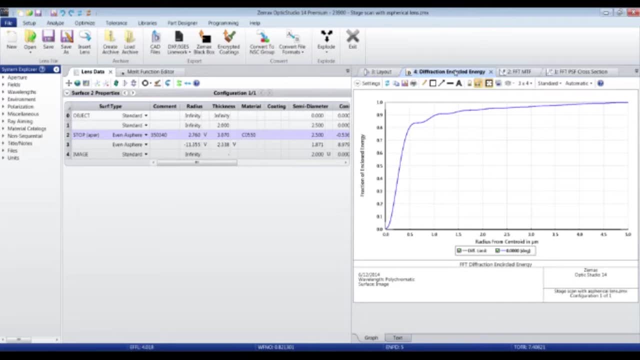 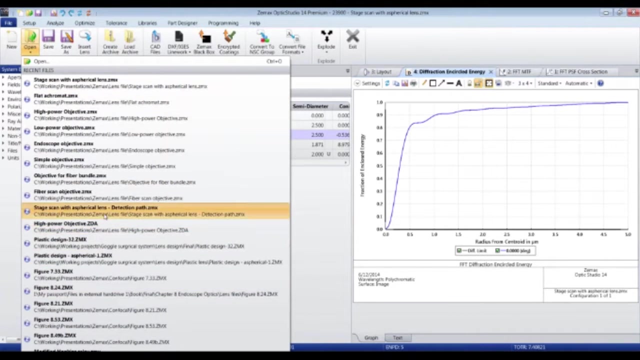 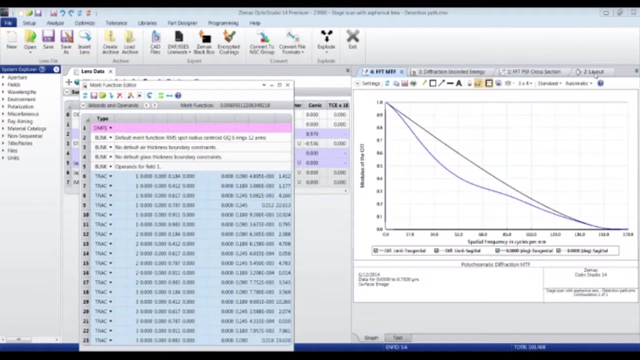 So for the detection, because it is used for confocal correlation image, So you need to work on a different wavelength. So the turbulence- W turbulence- is used to minimize the chromatic aberration. Here is the example. So, as you can see here, 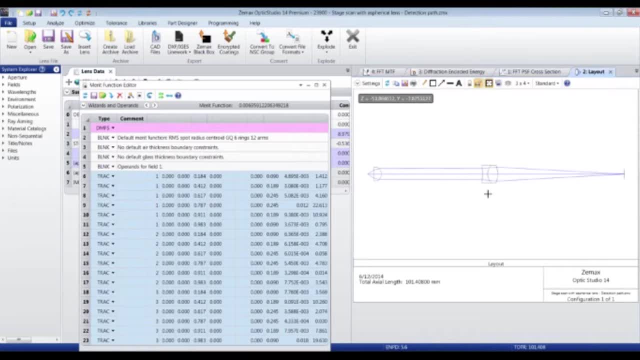 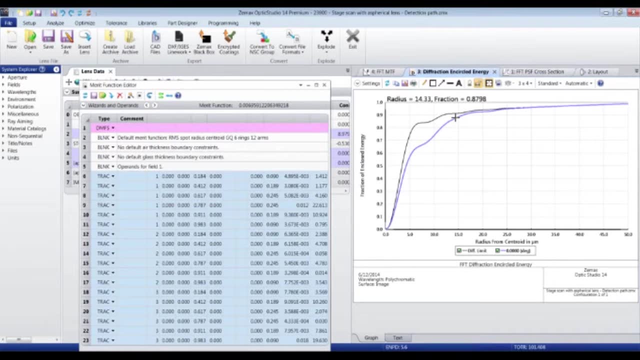 W is used to minimize the chromatic aberration. So, as I mentioned earlier, the deflection in cycle energy is very useful because you know your pinhole size, So you can estimate how much percentage of the light is within this pinhole size. 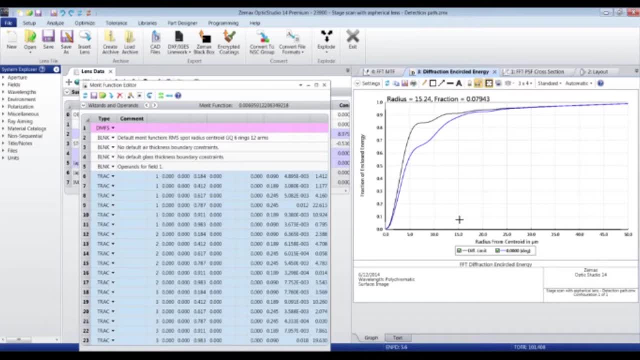 And also this in-cycle energy or in-square energy is useful when you design a system for CCT or CMOS imager, because that's the square typically. the pixel is square, So you can- you can change to the in-square energy, So that's a very useful feature. 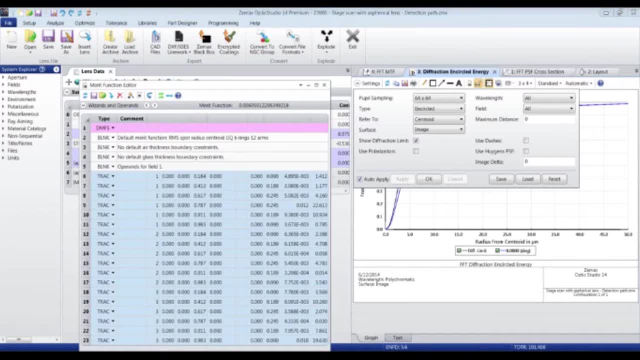 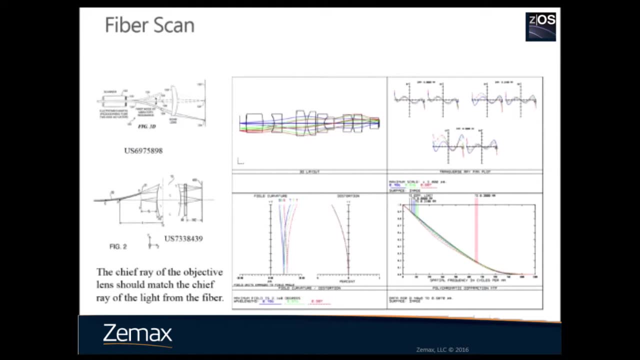 in confocal imaging system. So let's back to the presentation. So here is another example: the fiber scan. So fiber scan is not the red surface for fiber locus, It's not the red surface. So when you design this system, you need to know. 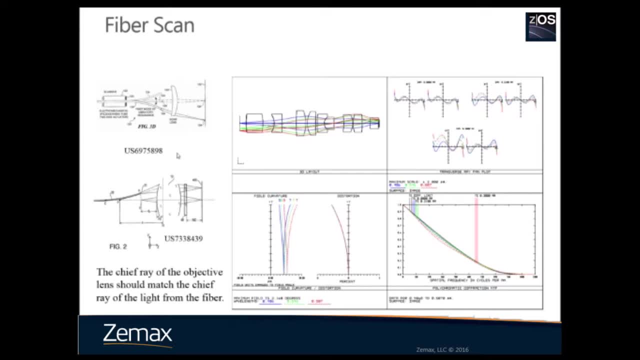 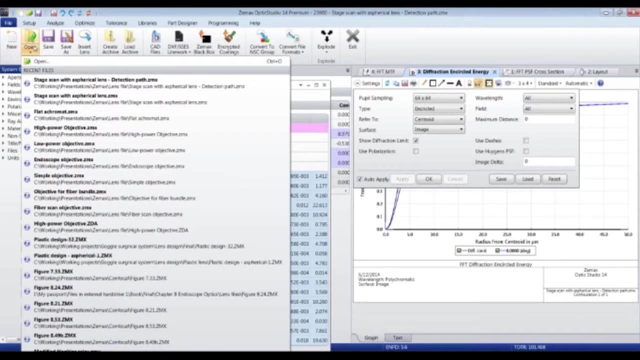 the radius of this fiber scan locus. Also, you need to control your chip rate. So the chip rate is like in the same direction as the fiber in each field of view. So let's see the example. So this is a very complicated lens. 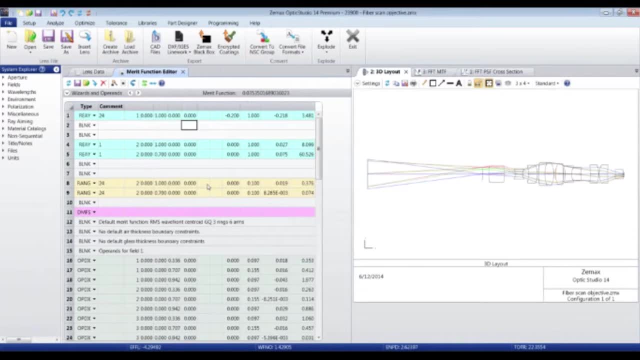 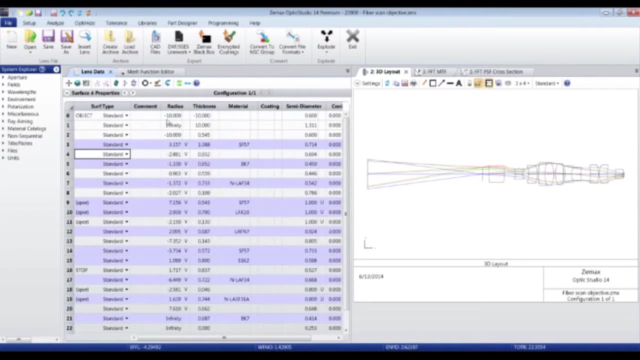 I use here only for to demonstrate the concept. For example here, as you can see here, the object is not black. As you can see here I put a 10 millimeter as the radius of this fiber chip. So also as you can see here. 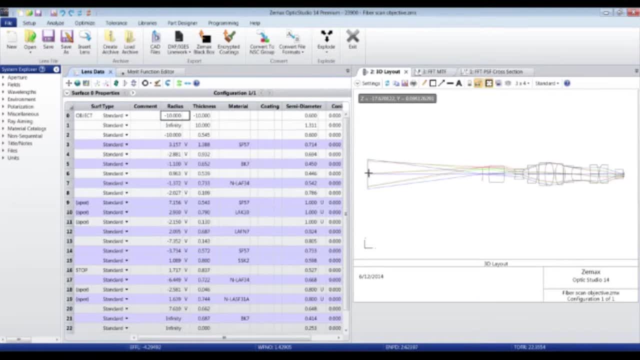 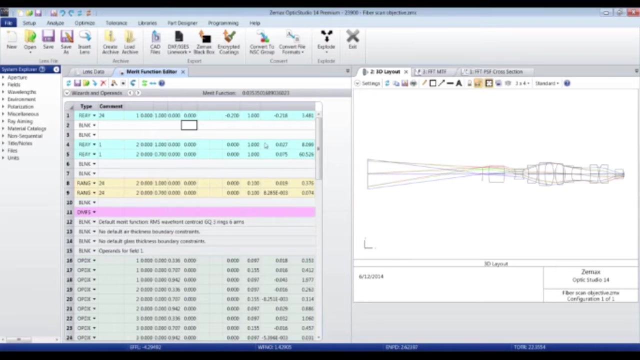 the chip rate is converged. the chip rate are converged to the pivot point of the fiber scan. So how to do that? to control that, you can put a dummy surface here And then in a magic function you control the rate high. 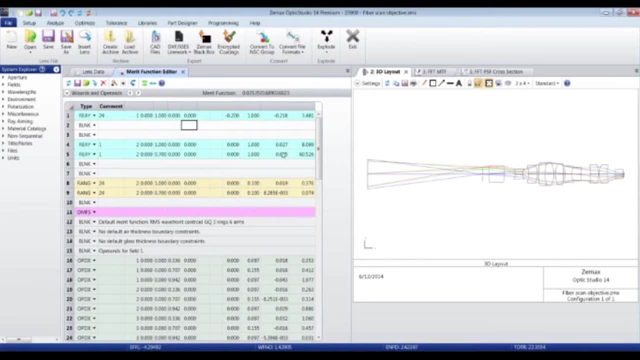 as you can see here. So you control the rate high here, so that each chip rate converges here, so that you can have the best performance in light efficiency. So of course this example is very, very complex, but I'll show you. 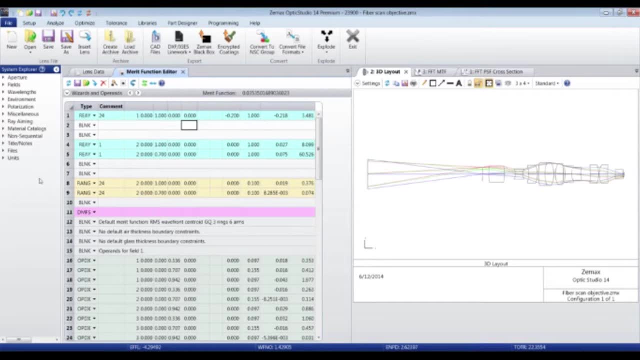 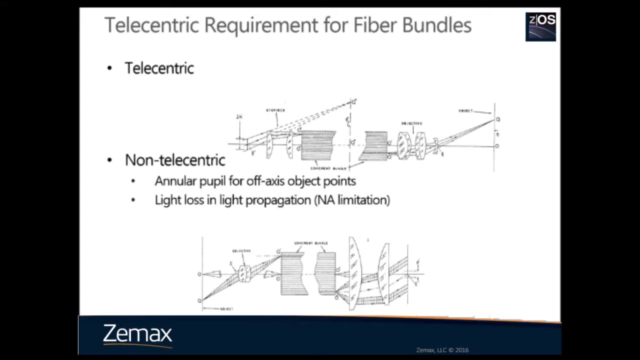 how to design a fiber scan system. Also, as you can see here, I also control the chip rate angle in the teacher's stuff. So that's another way to control the chip rate angle. And let's back to the presentation. So fiber bundle. 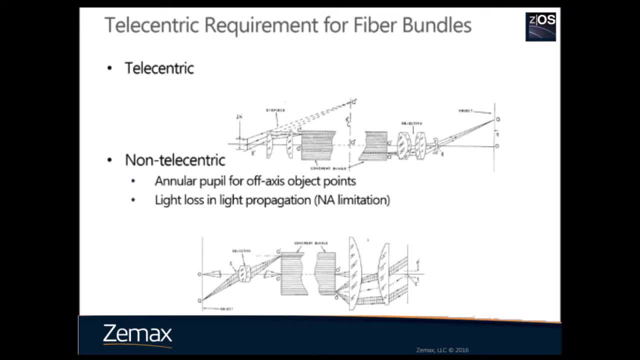 are commonly used in the endoscope- confocal endoscope. So what's different? What's the unique feature of the fiber bundle? So, for the objective you need to design as a telecentric image, You need to be able to see the fiber bundle size. 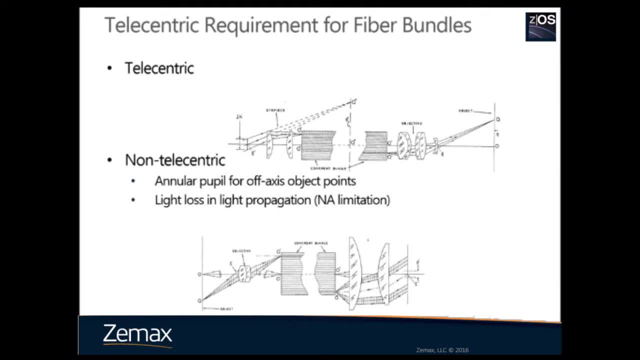 So if it is not, as you can see on this figure, the left line will couple into the fiber, And also there is no line in the center of the actual here, as you can see here. So just like on the system, 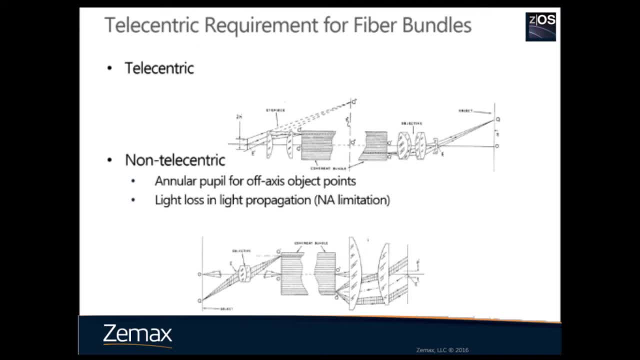 the center part is broken. It is broke So that your performance is staggered if you look at it from here. So there are two problems. if the system is not present, The left line is coupled into the fiber and the performance is staggered. 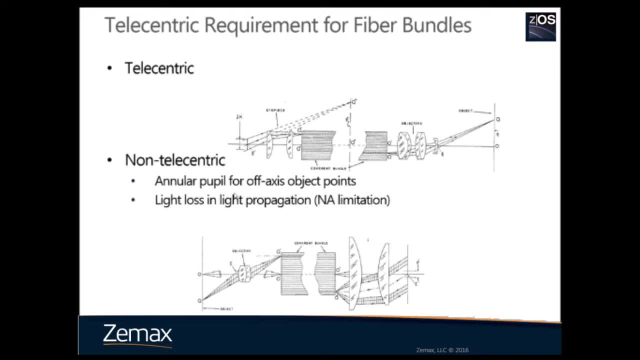 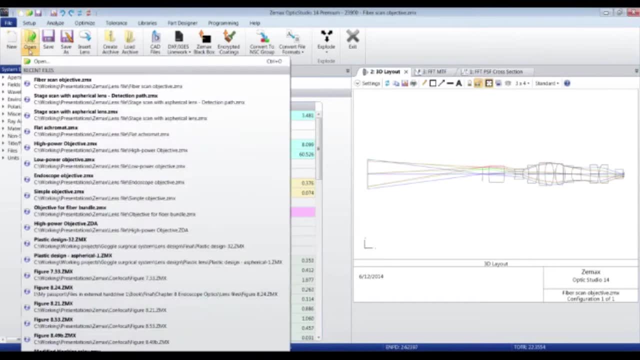 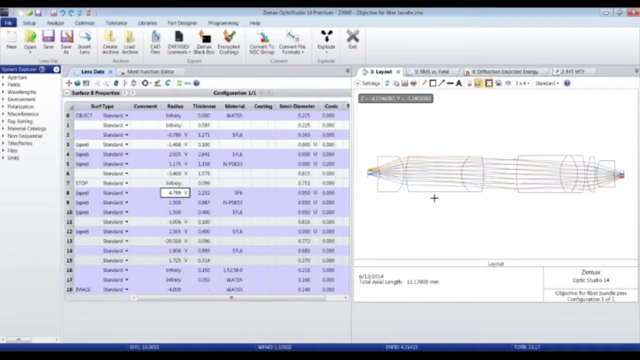 So that's telecentric. Telecentric is the requirement for the fiber bundle imaging system, And here is another example. So let's go to the CMEX. So here is the example of the confocal objective for fiber bundle system. So, as you can see here, 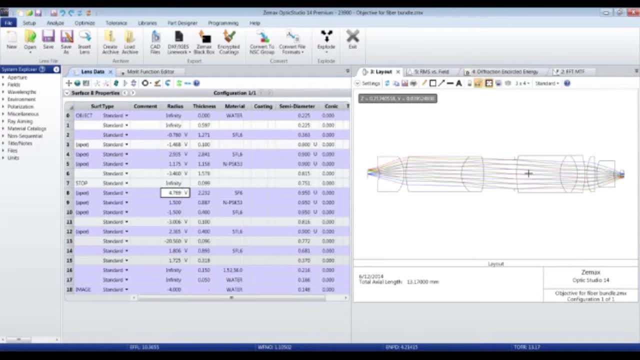 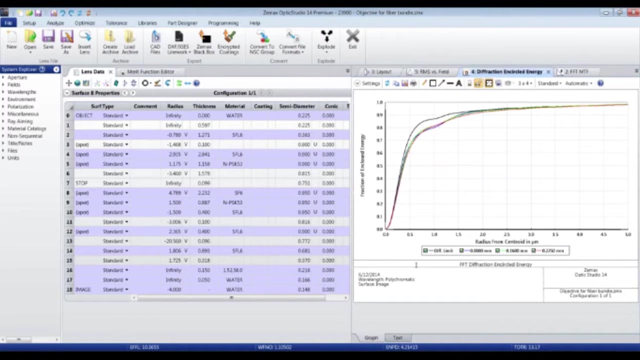 so it is more like a symmetry system. So symmetry system has an advantage because the operation on each half can be compensated- compensated to each other. Also, I used the in-cycle energy to estimate how the percentage of the energy inside the fiber, so you can estimate. 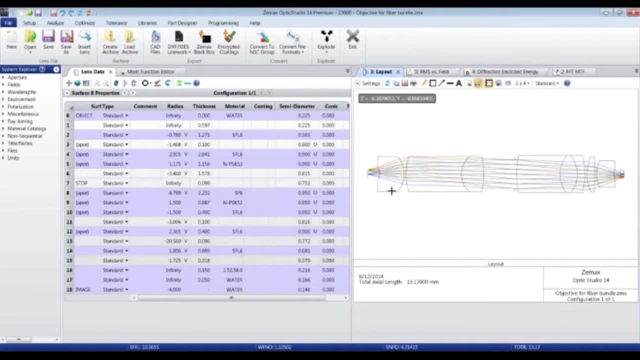 So, as I mentioned earlier, fiber in tissue size is better to have telecentric Because you scan inside the tissue. In the fiber side you also need to have telecentric to get a better performance. So this system is a double telecentric system. 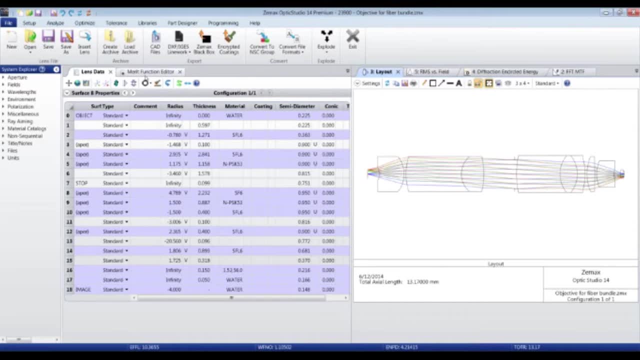 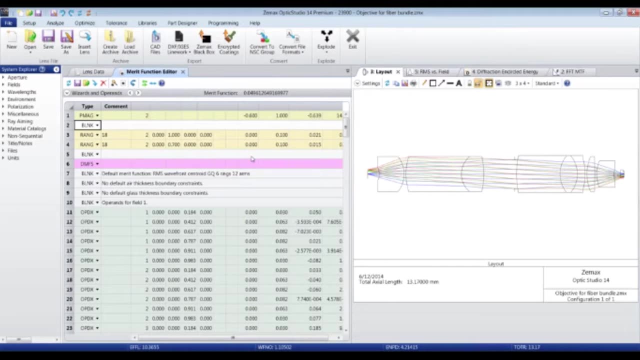 So in the imaging side I already showed that you can control the ray angle in a metafunction editor to minimize the truer angle In the object side. so you can specify here telecentric object space. This is how you can design a double telecentric system. 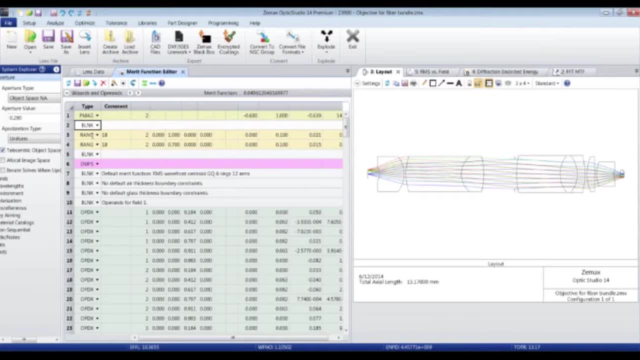 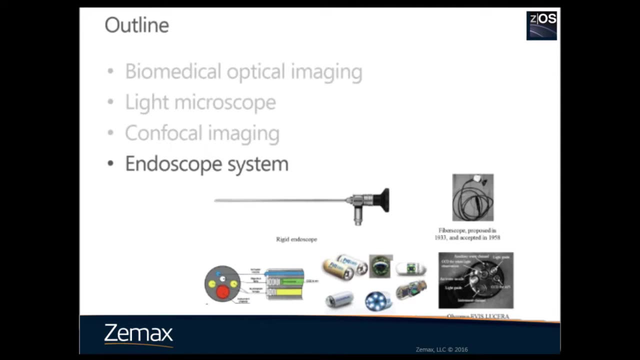 Of course you can control the tripler angle here in the object side as well. This is more convenient. Let's discuss the endoscope system. There are a number of endoscope systems, Like the simplest, the earliest, like rich endoscope. 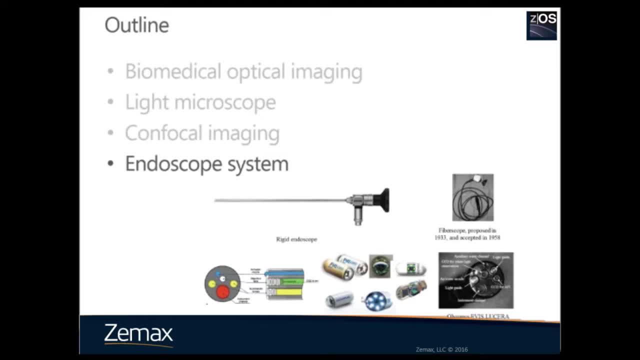 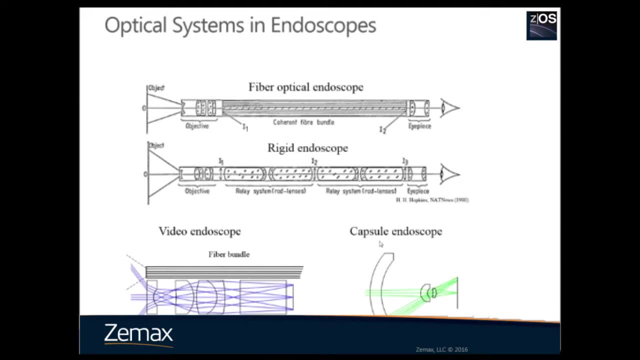 and then fiber endoscope, video endoscope and also the wide endoscope, the capture endoscope. So here is the optical principle. So for the fiber endoscope you need a fiber bundle to relay the image to the eyepiece. 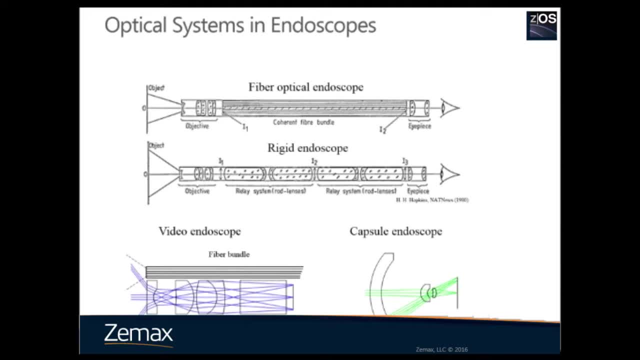 So we already discussed the requirement of a fiber bundle on the SIST objective For the rich endoscope. you can see there's a relay stage here. For the video endoscope the sensor is put on the distal end. You don't need a relay stage. 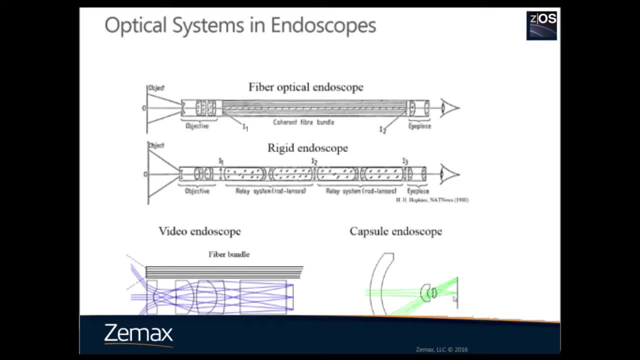 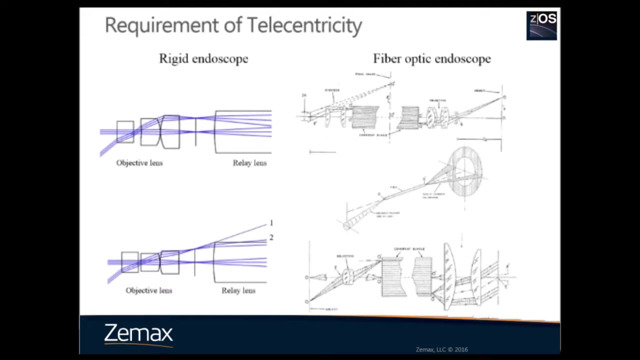 Capture endoscope. So here's the sensor. The system, as you can see here, is very simple, Not because the requirement is simple, because of the space. So here's the requirement on a telecentric system For the fiber endoscope. 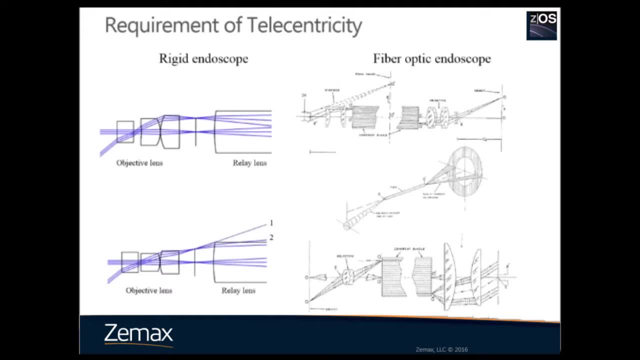 we already discussed, we need to have a telecentric in the fiber end. But for the rich endoscope we also need a telecentric system. So on the top figure I show the object is telecentric. So all the light. 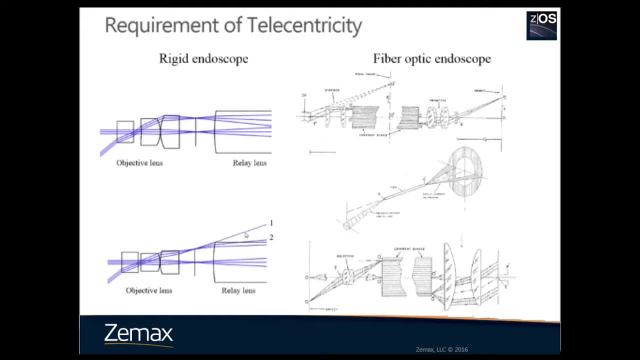 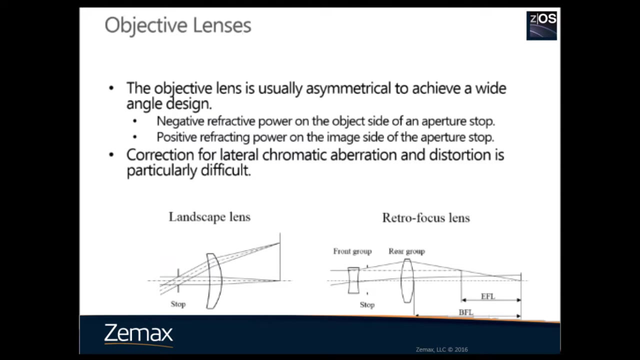 will couple into the relay lens. If it's not so, as you can see here, some of the light cannot enter the relay lens After several states, so your performance will be like a significantly So for objective lens in endoscope, because it's inside the body. 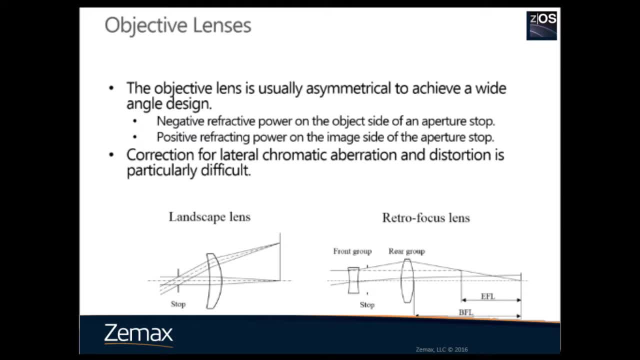 so you want to see as large area as possible, So typically your view is large, So that means you need to use either landscape type lens or lateral focus. So one of the common problem for both systems is the system is not symmetry. That means collection of. 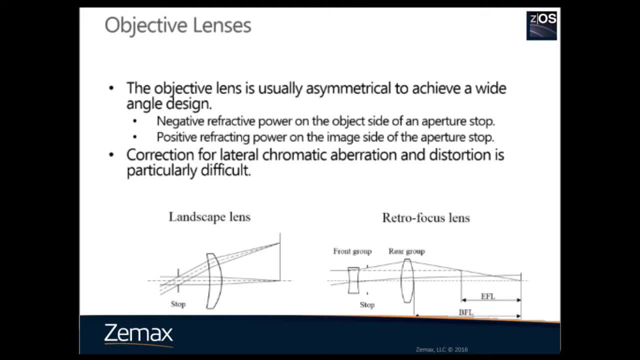 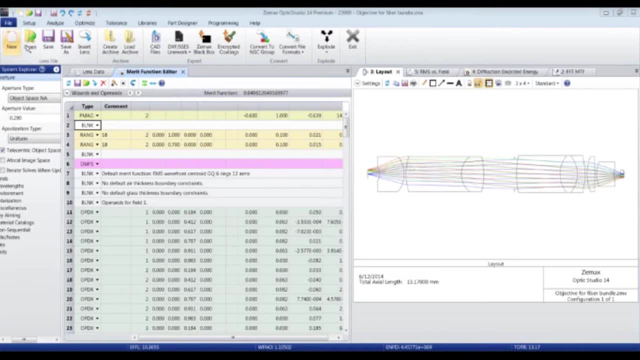 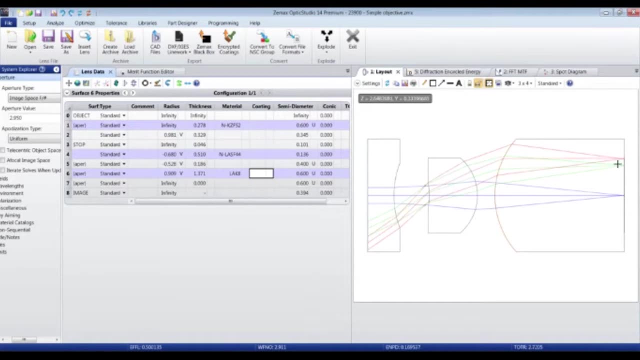 lateral chromatic aberrations, distortion and coma is more challenging. So here is one of the example, So very simple example, So I'll show you here. So it is designed as a telecenter in a fiber bundle space. So the reason: 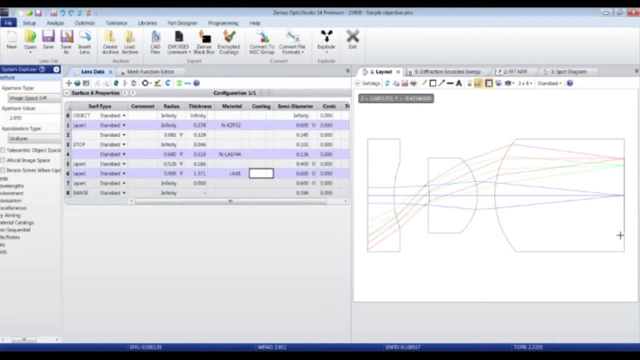 one of the reason to put a limit lens on the surface of the lens is you can attach the fiber bundle to this lens, So you don't need to control the distance between the fiber bundle and the lens, So you just put it there. So, as you can see, 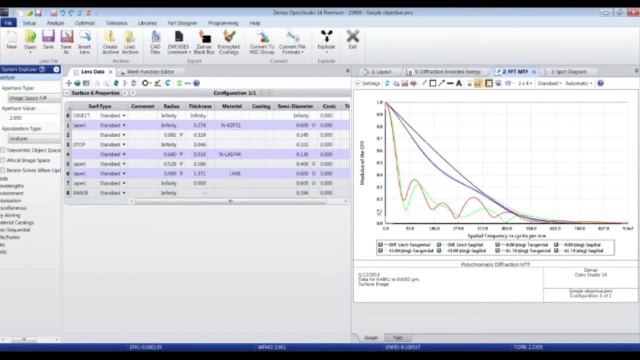 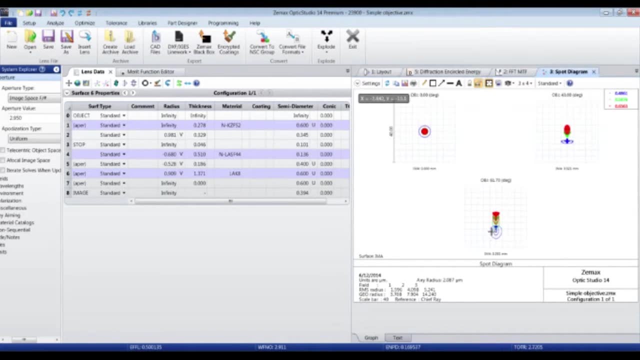 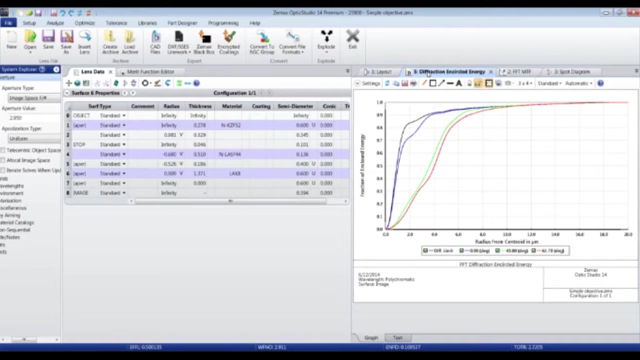 the performance is not very good. So because you told the aberration value earlier and also from the point like a spot diagram, there is a significant lateral chromatic aberration. So if you need, here is another like a tool you can use to estimate. 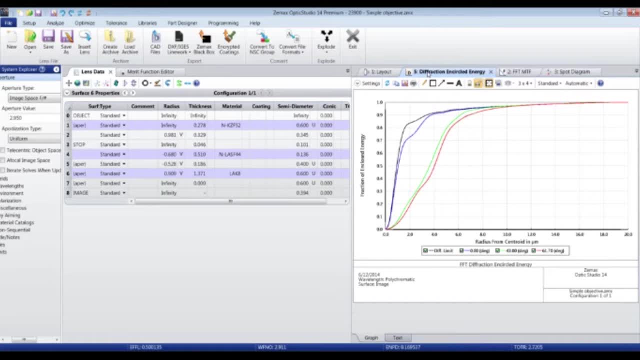 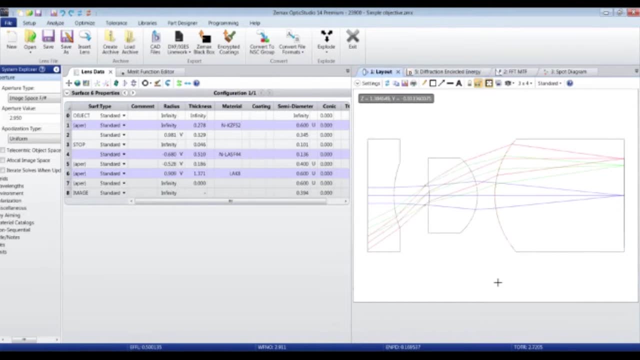 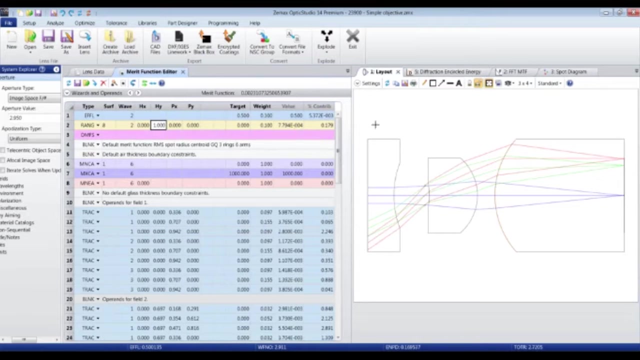 how the percentage of the energy inside the fiber. So the performance is not to actually discuss the understanding because it only is a three-singlet here. So also, so we control the triple angle in here. So you can see the triple angle is smaller. 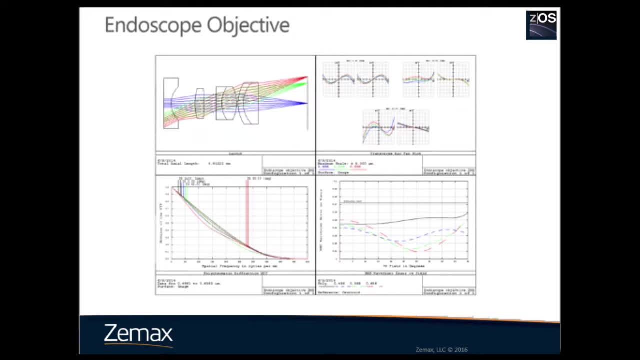 is small. So in order to increase the performance you can add the cement debris to reduce the chromatic aberration And also you can add more elements in the ground group. So the system is more cement, so you can compensate the aberration. 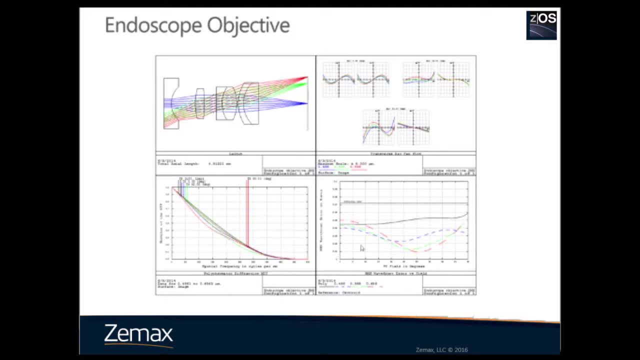 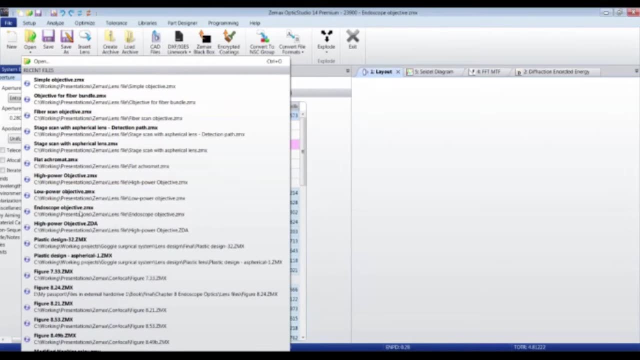 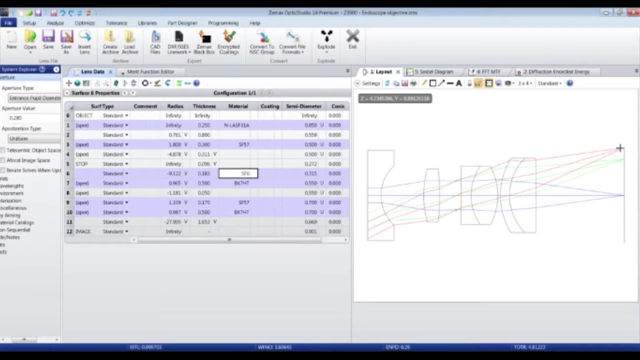 As you can see here, this objective has a much better performance. So here is the cement example. So, of course, as you can see here, the chiefly is angle is not. it's not telecentric, So it cannot be used. 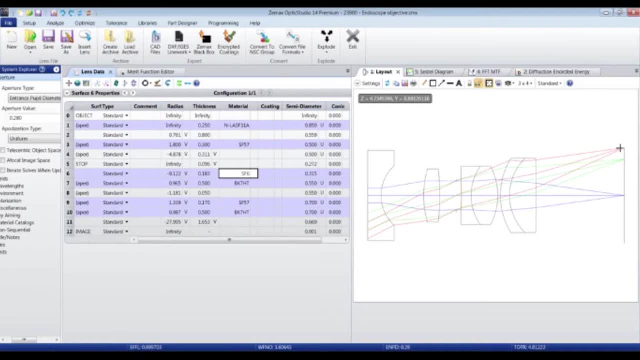 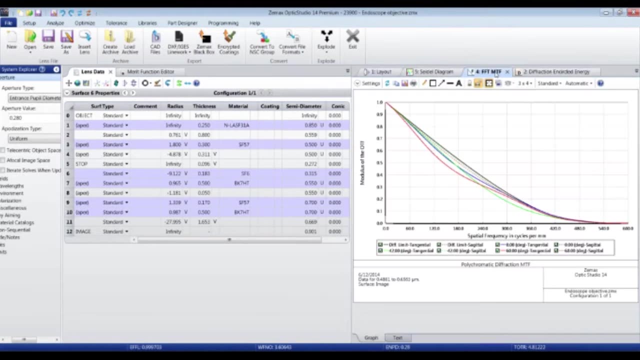 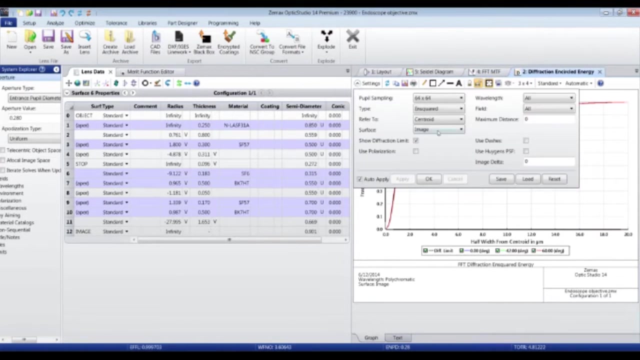 for rich endoscope and fiber endoscope, So it can only be used for the video endoscope or CMOS here, As you can see from the performance, it's much better So for this case, because it's CMOS, so it's better. 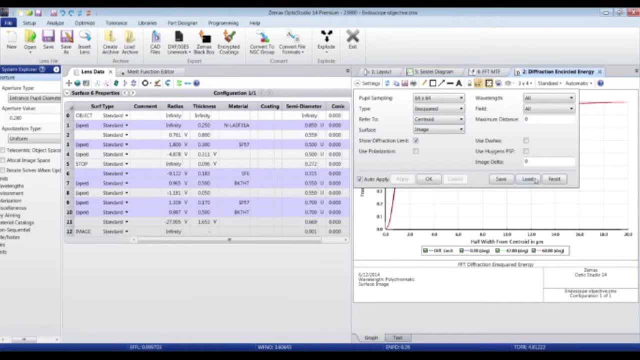 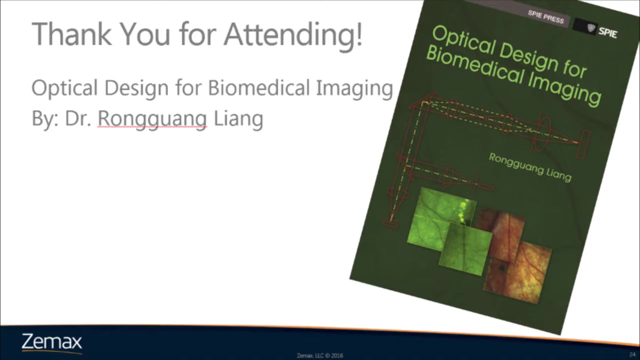 to change to the N-square, N-square energy. So you know the percentage of the power in each pixel. So, as I mentioned earlier, you can see it's much better than the N-square, N-square energy. So, as you can see, here the 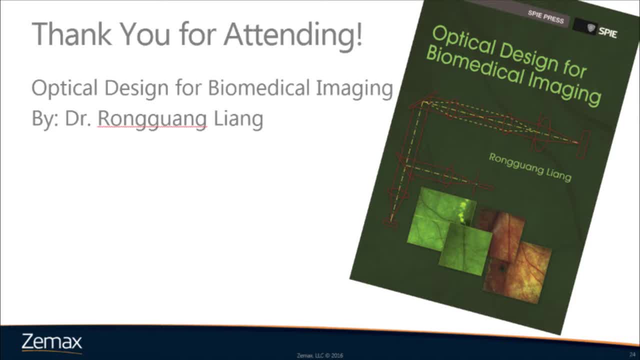 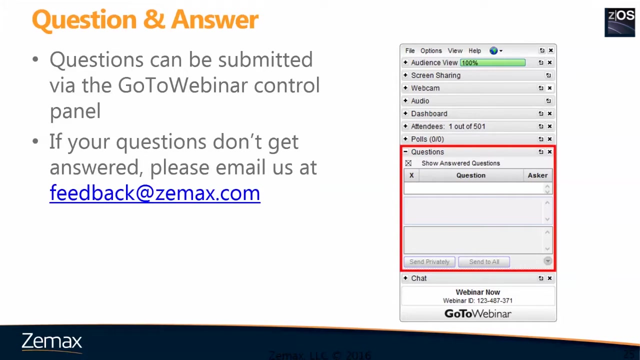 N-square energy is much better than the N-square energy. So, as you can see here, it's much better than the N-square energy. So here is the N-square energy and the N-square energy. So, as you can see here, 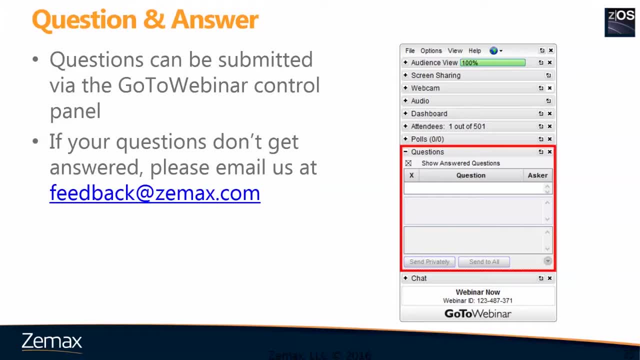 the N-square energy is much better than the N-square energy. So it's much better than the N-square energy. So let's see what we consider for the tube lens and the microscope design. So constraint is first the wavelength. 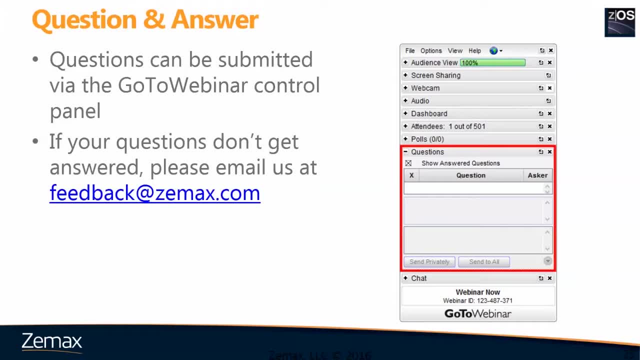 the spectrum. So if you're looking for single wavelength, so that means you don't need to minimize the chromatic resolution. So, of course, if you want to improve the performance- for example like to achieve a high image extra- 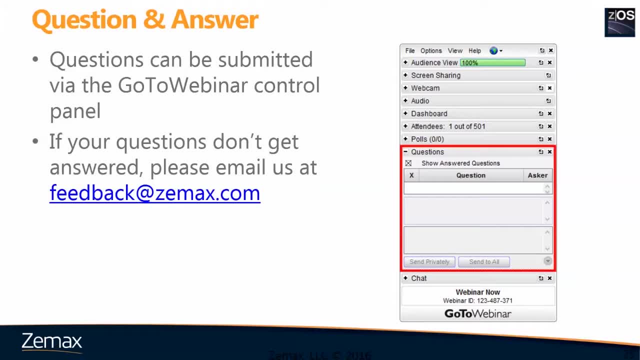 you may use, for example, like a CTU and the objective in the CTU So you can have like a radical. they can only like read on on axis. So if it is of axis the performance decorate significantly. So the constraint. 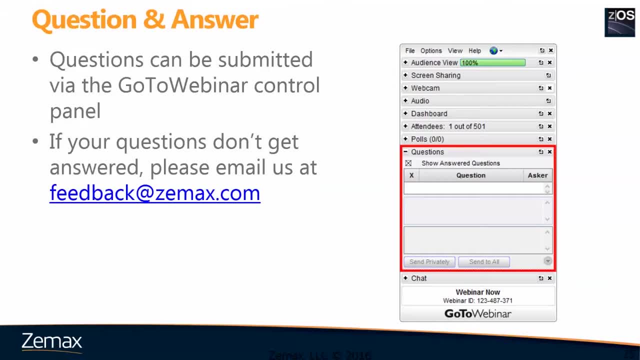 all depends on your requirement. We'll cover here ablation control and walking distance and space limit. So if you have any questions about the design constraints for the capsule style of endoscope, are there any special constraints on that one? Yes, So. 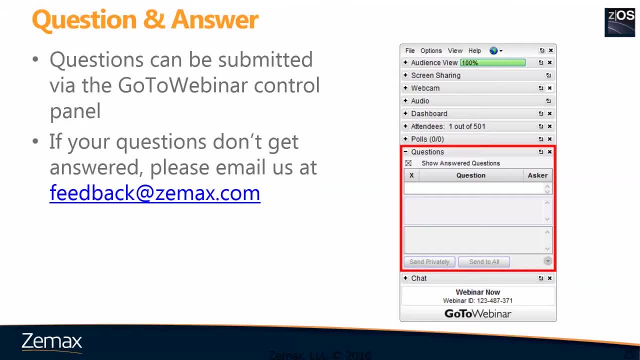 that's very unique. So I have- because the I can see- go back to here So you can see this is a dome part of the object system. LED is here, So let me see. you need to configure the reflection, the illumination. 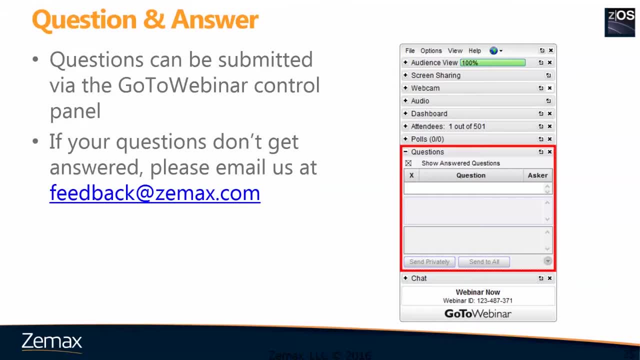 from these two lights. So just like you inside a house when you turn off the light and then you want to capture the street outside with just a flashlight, So most unlikely you couldn't get a good image because the reflection from the light is. 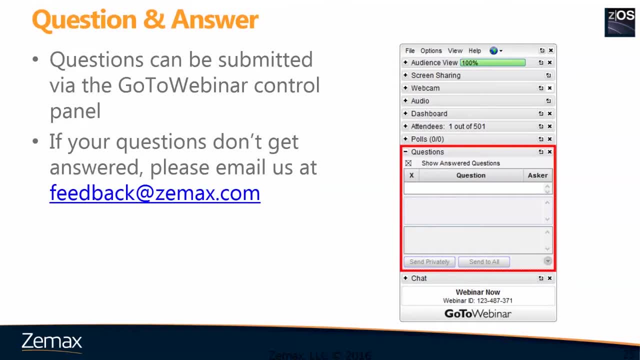 very small, So you can see that the reflection is very small. So you can see the reflection from the light and the reflection is very small. So for the reason it's lightweight and it's much low cost, because once you have a 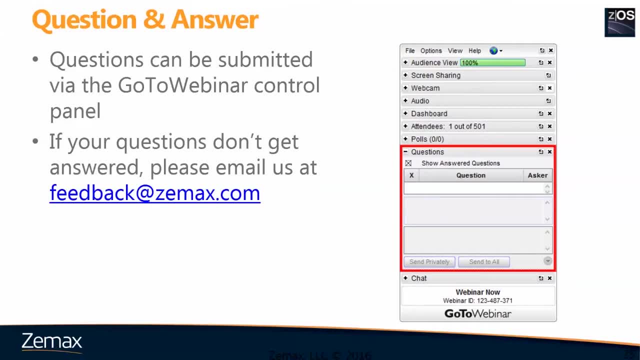 mold made, so the lens is very, very low cost, maybe less than one dollar or less. so there are much less choice in plastic elements. Also, you need to consider the first element because, for example, endoscope, your first element always contact with water. So 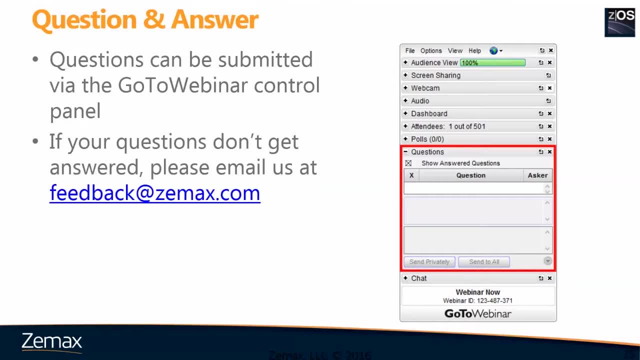 you need to select a plastic material to fix the plastic material and then you need to go to the next element to fix the plastic material So you can choose. the plastic material is different, or if your index is different, So you can use a multi-configuration. 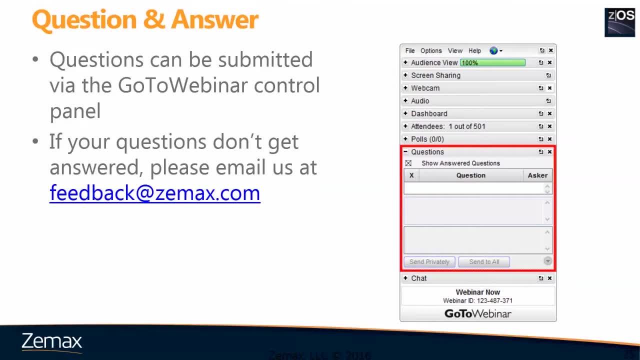 So you can see here. So where is the multi-configuration? So that's something you can use as a multi-configuration system. You could optimize the OK. excellent, Thank you for that. Here's one. Is there a good way to avoid back reflection from the lens? 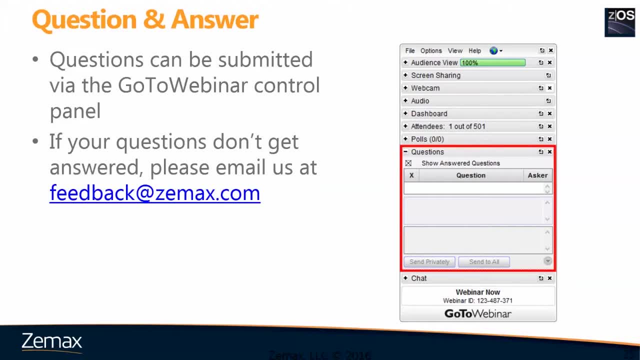 surface in your design. The simplest is to use the AR coding. So, like I said, a very good coding. Of course you could do the analysis. That's one of the functions in ZMAX. You can do that to find out which. 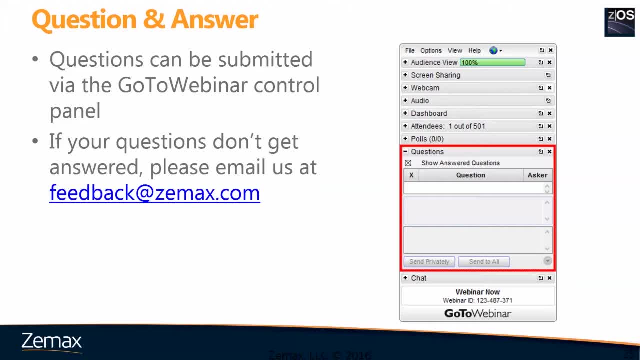 surface is the most visible, Like most of the ghost image, or the best reflection, And if you locate that you could change your coverage, So another way to do it. so that's the camera. So once they locate which surface, which portion, 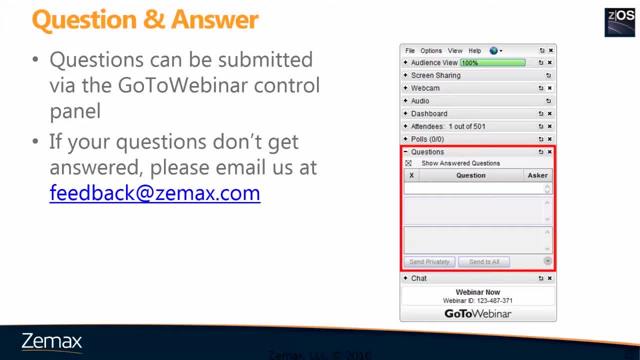 is the best reflection. they put a small black box there, So that's to reduce the back. OK, So it's a case by case. OK, excellent, Got a couple more questions here For the objectives in the fiber optical endoscope. what is the typical size? outside diameter Depends, For example, fiber bundle usually is a couple. The lens is a little larger, like 3 millimeter. I see the 2 millimeter objective because all depends on the field view. 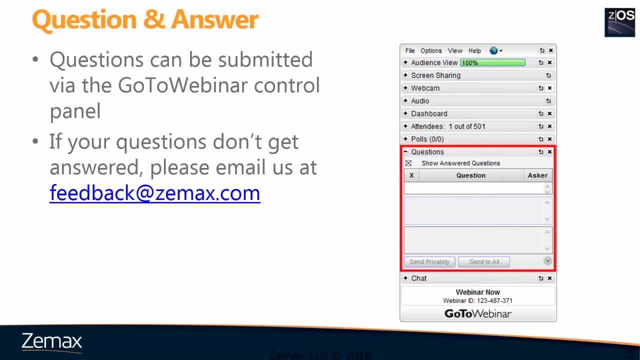 So If you want to have a large field view, your lens has to be larger. If you can find your field view, you can reduce your objective, your objective. So 2 millimeter to 5 millimeter is feasible. So if you want to go to 1 millimeter, 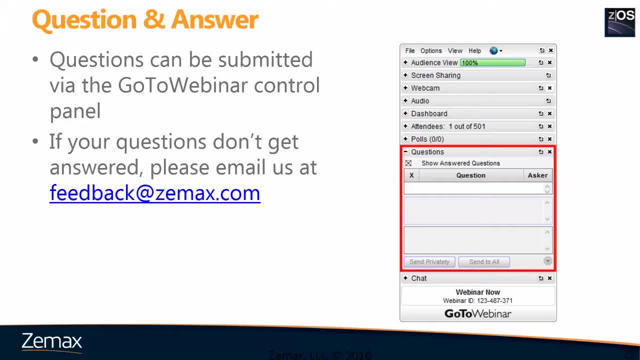 then you need a lot of effort. OK, excellent, Thank you. Here's a follow up to the lens reflection question. With two reflections, Is that generally acceptable? Hard to say Depends on what percentage, For example, if you have one you. 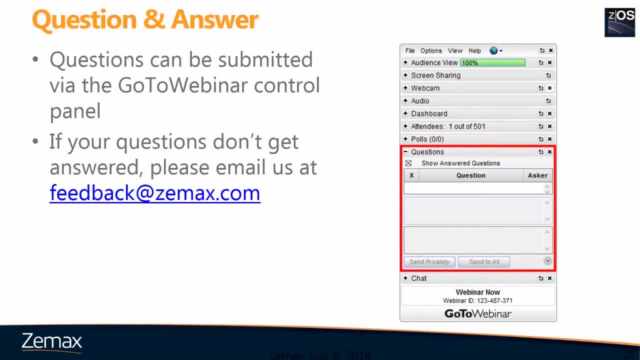 might have one reflection, But your reflection is very small compared to the image. That means you blow your image. Even if it's one reflection, your objective is useless. So for another case, if you have 10 reflections, 10 very tiny- 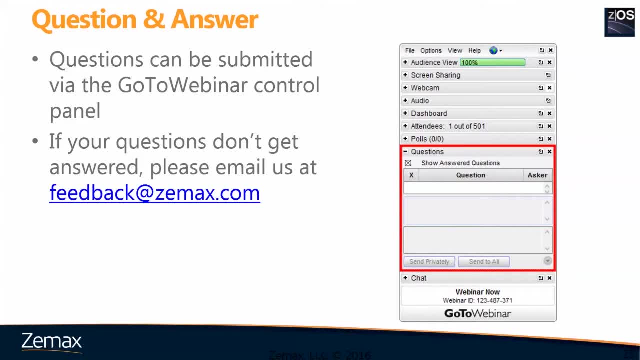 even if you see the reflection but the percentage of the image is very small, then even 10 or more is not an issue. All depends on the relative. Like a drone, for example, how much percentage, how many percentage of the light relative to your image? 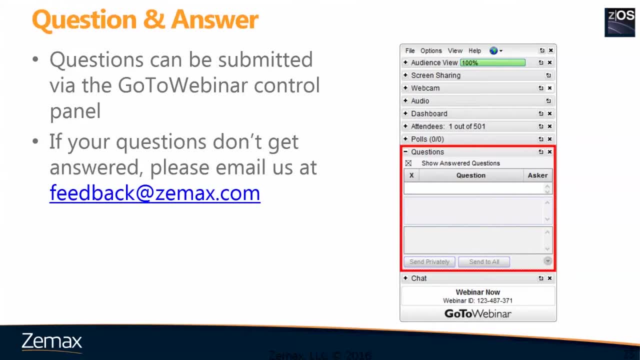 OK, excellent, Thank you. Here's another question about modeling tissues in ZMAX for absorption diffusion. Are there existing models? How do you actually model the tissue? That's a good question for you. You're saying how to go answer here. 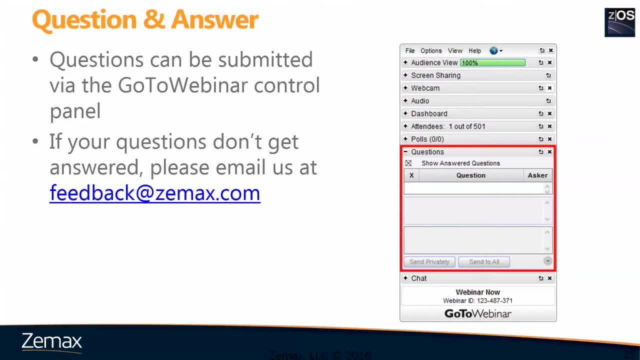 For the illumination side, for example, once you know the tissue property you can build a stature. What is better? illumination function in ZMAX. So that's one way to do it. So I did not do it. I did it in like a simulator, like tissue scattering in ZMAX. 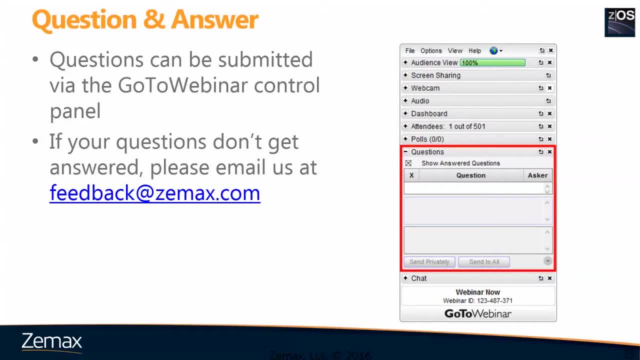 So I don't have a good answer. Maybe you guys in ZMAX have a better answer. OK, we do have some models in ZMAX to help us with tissues to model them, But it is a very, very difficult science at times. 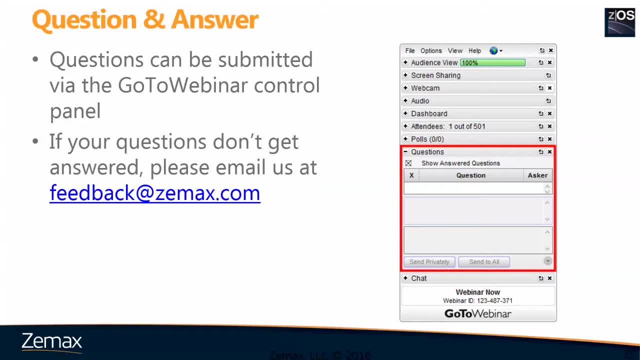 Here's another question for you about the proper NA in objective lenses, since it relates to the depth of focus. What is the proper NA? What is the proper NA for your objective lens? So it's a very broad question, So we need to know what application. 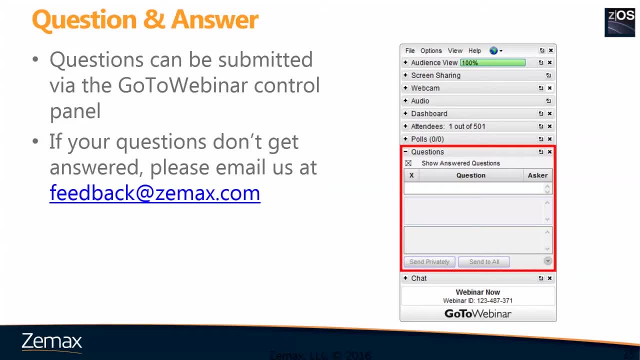 Is it like a microscope objective or is it like an endoscope? or it is an objective for OCC or for a fluorescent image. So it depends. So NA, for example, for a fluorescent image. you don't really actually want to have a large NA. 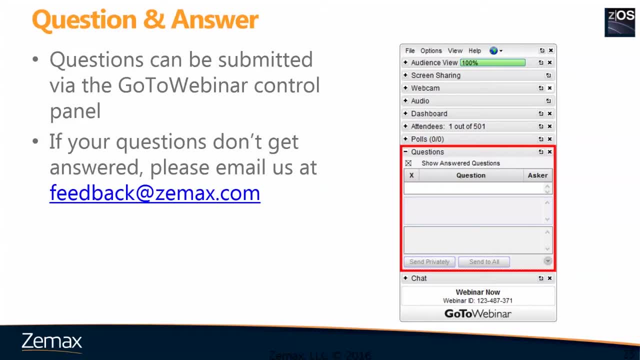 for fluorescent collection, But with the limit space or limit like theater. probably you want to minimize abrasion for that NA, But if you don't care about resolution, you care more about the fluorescent collection, so you can increase the NA. 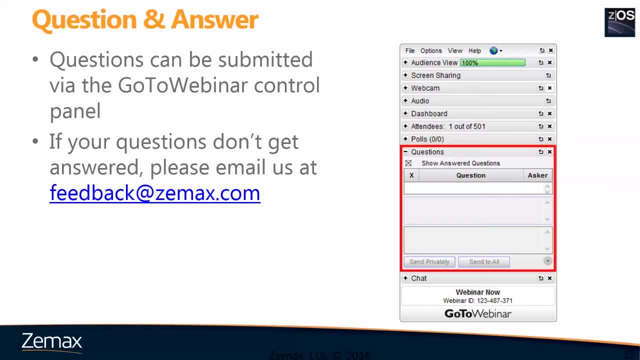 But if you really have a good resolution and then you have to care for when you increase the NA, because the signal is not good enough. So the focus will be more complicated. That's the field, That's the focus will be smaller. 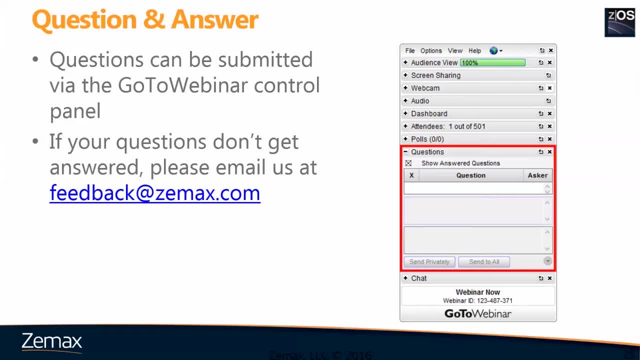 But for the fluorescent, maybe for tissue image, probably that is not really important. So it all depends on your requirement. What application? So that's very difficult to answer if we don't know what is the application, what is the requirement. OK, good. 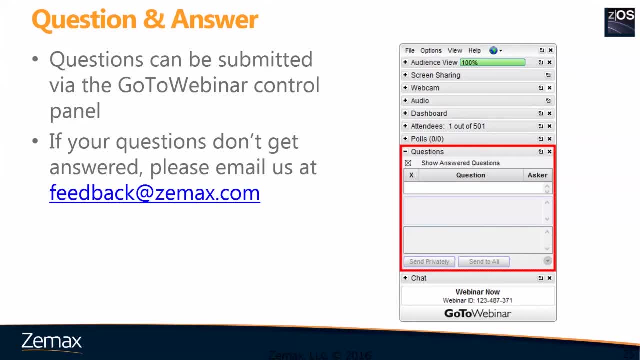 Thank you. Now here's one. It's more specific. They're looking for suggestions for lens systems for OCP imaging with a working distance of around 300 millimeters, for minimizing abrasion and field curvature. So they're just kind of looking for suggestions. 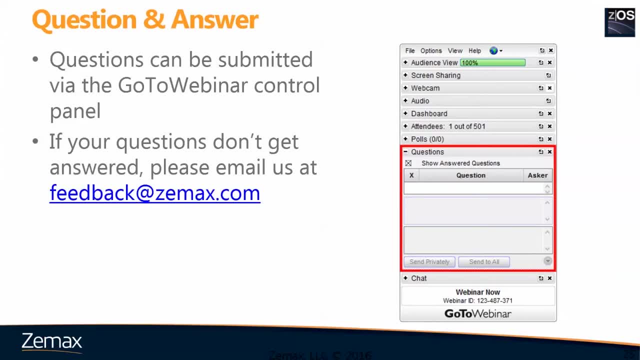 for lens systems, OCP, usually your NA is not large or you're 0.1.. So I think that would be sufficient. OK, excellent, That was a good one. Here is one last question. It looks like on the manufacturing. 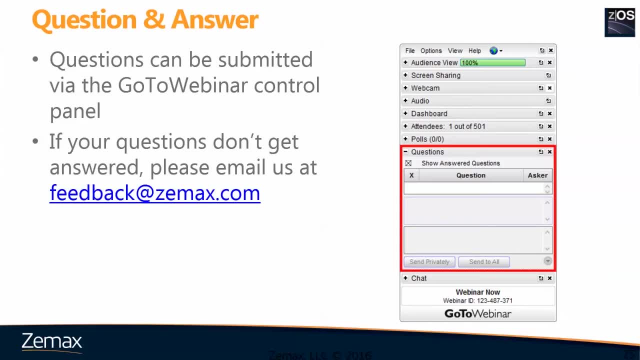 that maybe you can help us with. they have an objective with many cemented acromats. If the OD is 2 to 3 millimeters it's challenging to manufacture. So what's the low limit for outside diameter for manufactured cemented acromats? 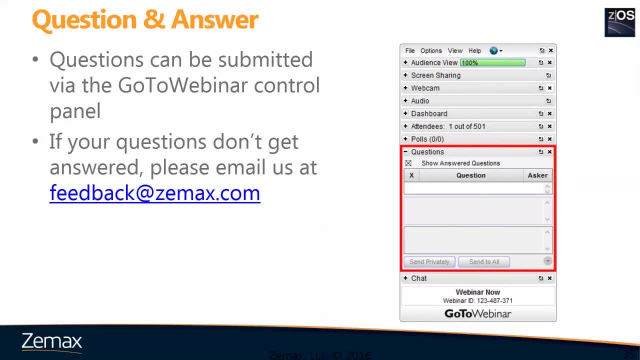 I see the 0.8 millimeter. I see some companies can make it as small as 0.8 millimeter, But of course there are And manufacture costs will be very high. Oh yes, good point. Well, thank you Ron. 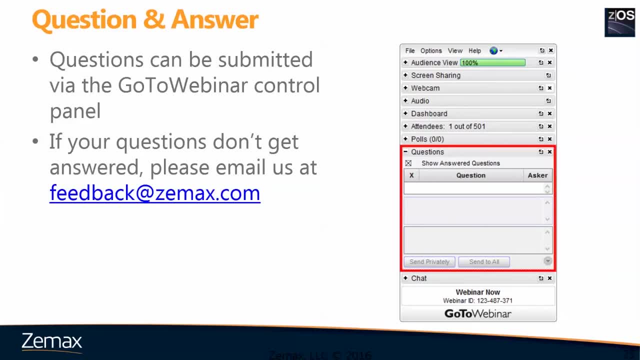 That looks like all of the questions we have. There is one that just jumped in, So we'll handle this. one last question And then we'll have to call it a morning or afternoon, wherever you may be. Do you have anything special to minimize spectral effects? 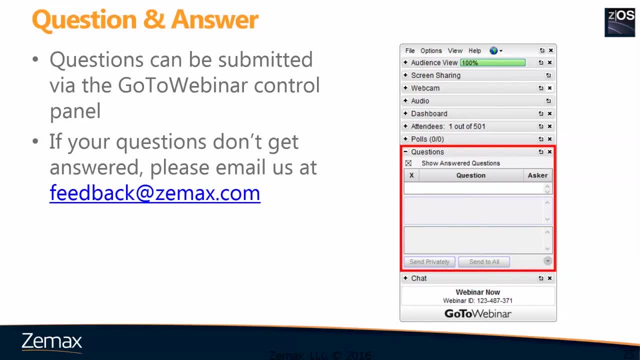 when using a laser. This is not what you can do in a lens design, So you have to. You have to manipulate your light source. Either use rotating scatter plate and to minimize laser, to reduce cortical length, So also you can use a low cortical light source. 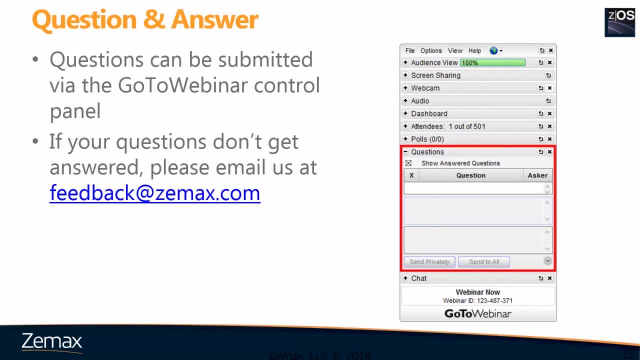 for example, like a broadband laser source. So if you have a cortical laser source, only way you can do it is to use the cortical length before the light is launched into the objective. So nothing we can do in the objective, in the lens system. 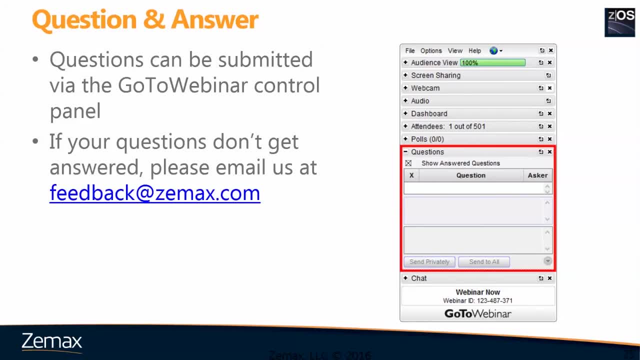 OK, excellent. Thank you very much, Ron, And it looks like all the questions we have today And thank you very much everyone for attending. If you have an additional question, you can go to support at zemaxcom And we can try to help you out there.